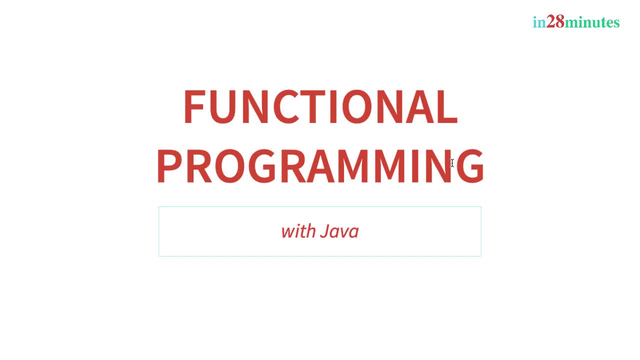 like REST API frameworks like Spring Boot and front-end frameworks like Angular, React and Vue. I have been programming with Java for more than a decade and a half And I have been using functional programming with Java for the last few years. In 28 minutes, we ask ourselves one. 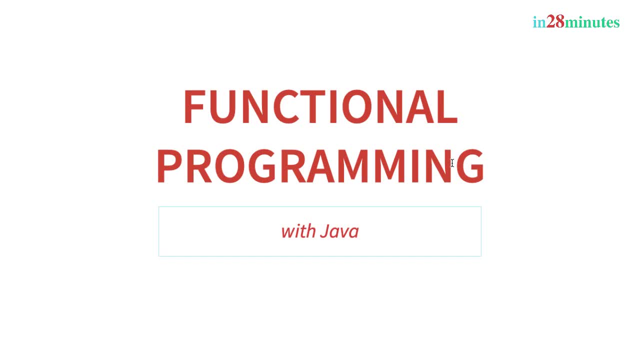 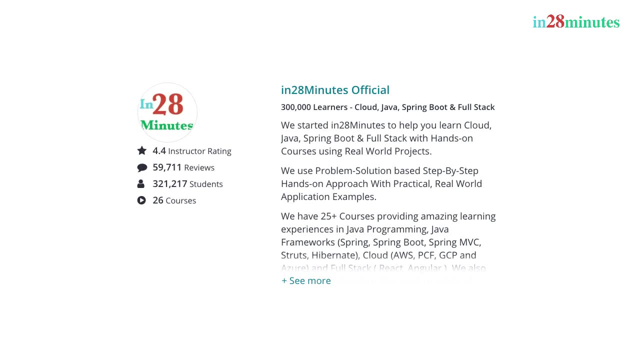 question every day: How do we create more amazing course experiences? The success we had on a variety of platforms, including Udemy, with more than 200,000 learners, is a result of this pursuit of excellence. We love programming and we believe that learning. 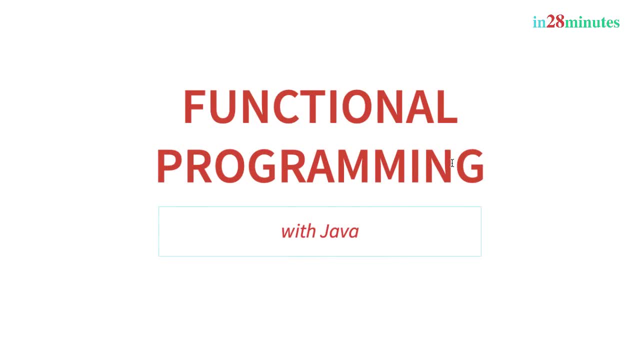 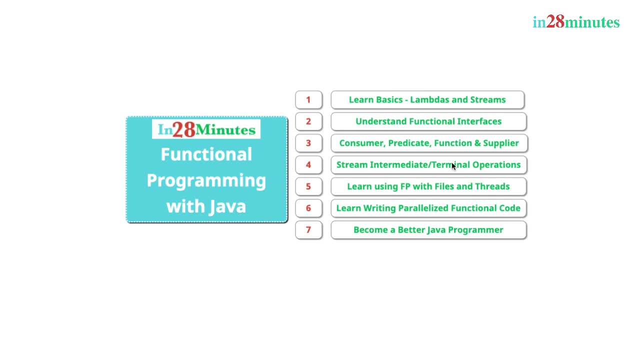 functional programming is one of the essential skills for Java programmers today. In this awesome course, we'll help you to learn the basics of functional programming. We'll help you to learn lambdas, streams, different functional interfaces like consumer, predicate, function and supplier. 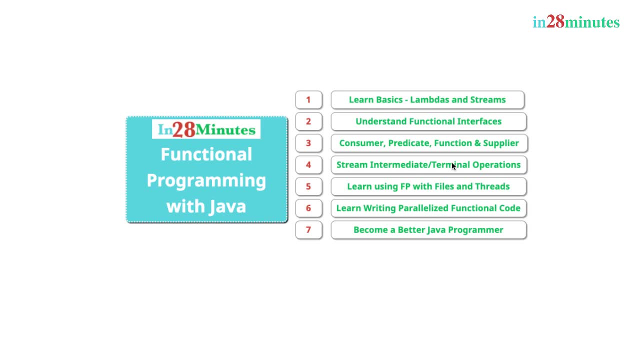 We will look at all the different operations that you can do on streams. We'll look at how you can use functional programming with files and also threads. We'll help you to write great Java code using functional programming And we'll also help you to learn how to. 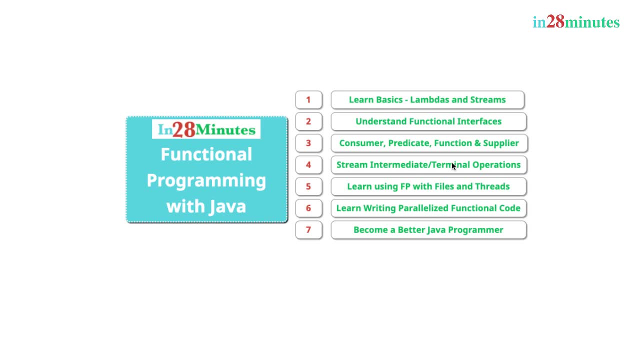 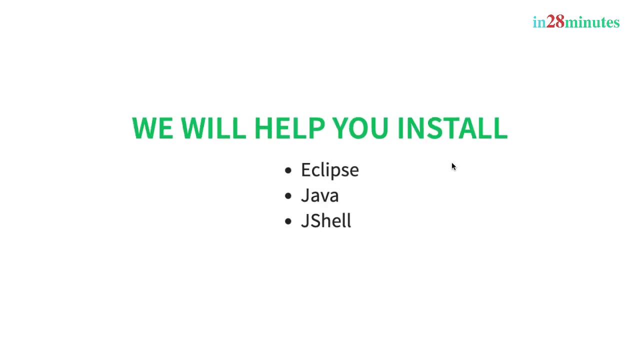 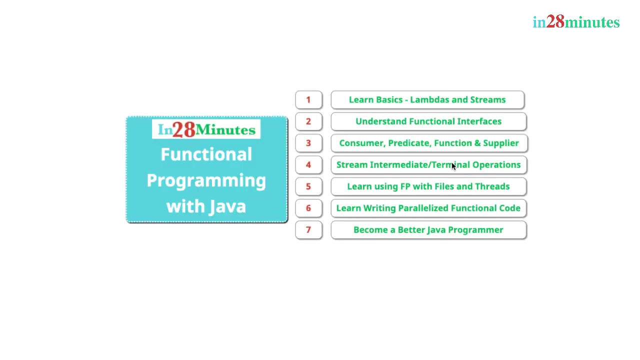 write performant and parallelized functional code. We expect you to have some experience with object-oriented programming in Java. We'll help you to install all the tools that you'd need for this specific course: Eclipse, Java and JShell. The complete source code, including the step-by-step details of this course, are available on the GitHub repository of the course. 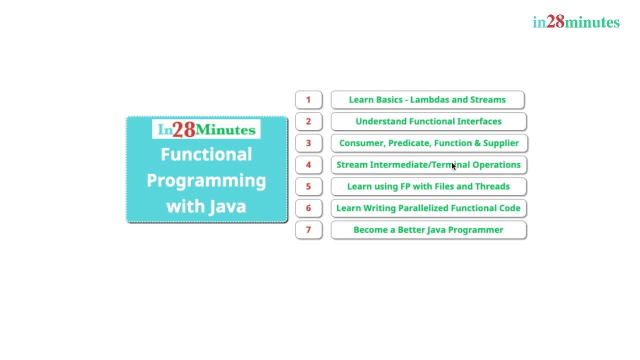 What are you waiting for? Let's have some fun learning functional programming with Java. We had a lot of fun creating this course for you, and we're sure you'll have a lot of fun too. If you want to learn more, go ahead and click the enroll button, Or you can take a test drive by using the free preview feature. 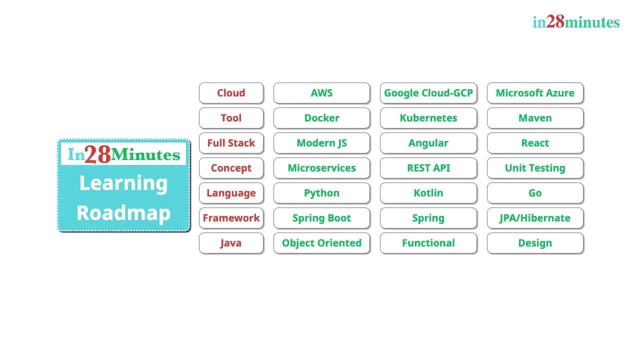 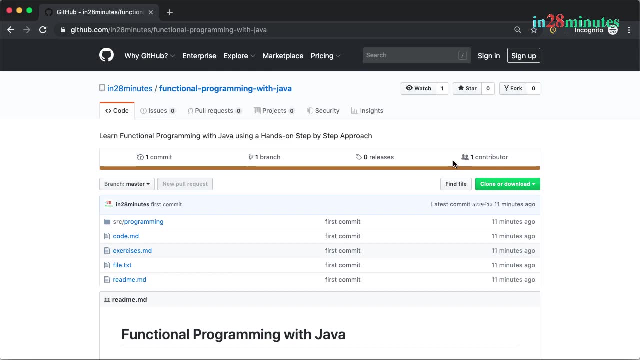 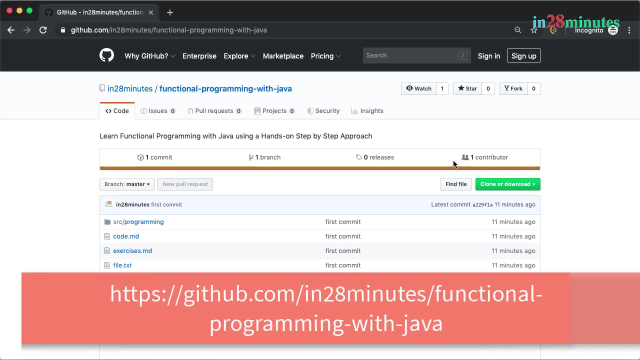 Good luck and I'll see you in the next video. Welcome back, Congratulations on making a great choice in choosing to learn with this course. In this step, let's get familiar with the GitHub repository of the course. One of the first things that we would recommend you to do is to bookmark the GitHub repository of the course. 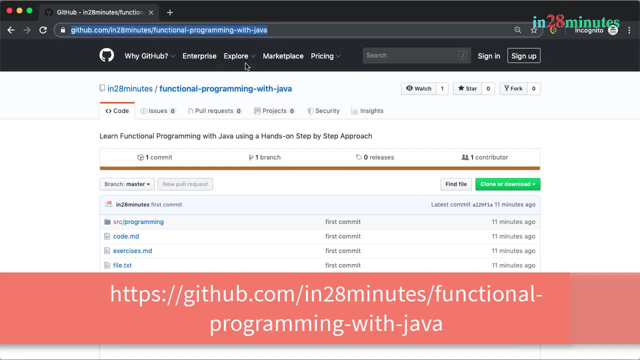 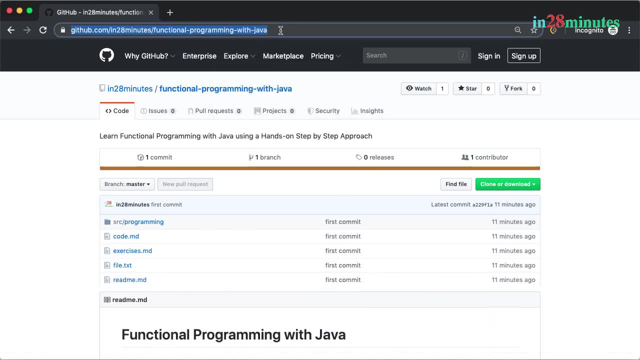 The GitHub repository of the course is githubcom. slash- in28minutes- slash- functionalprogrammingwithjava. You'll also find a link to this in the description. You'll also find a link to this in the resources section of this specific video. The GitHub repository contains all the information that you would need to complete this course successfully. 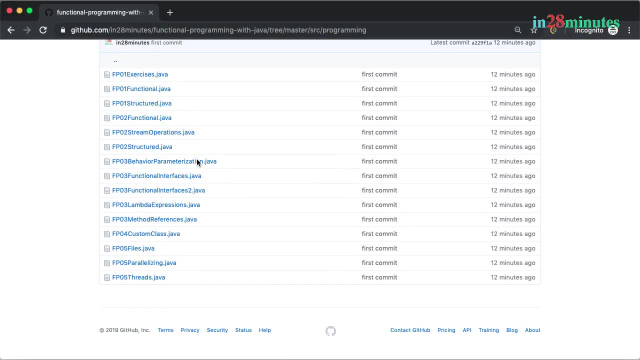 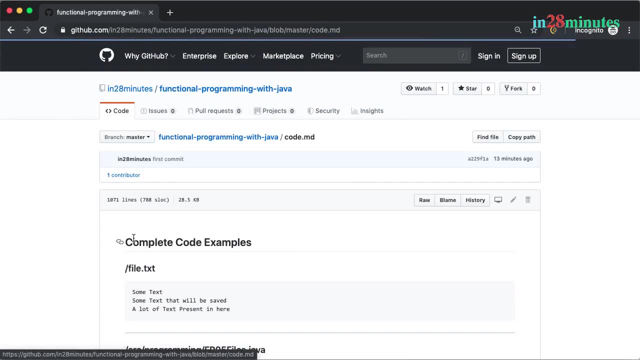 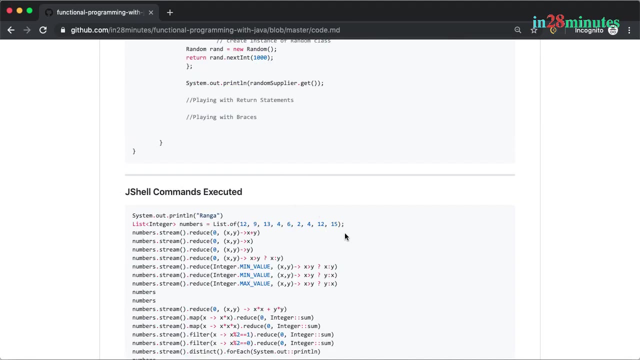 The source slash programming contains all the Java files that we would be writing during this course. In addition to this, we also have a codemd, where you have a listing of all the Java files that we would write during the course. The code file also contains all the code snippets that we would execute in JShell. 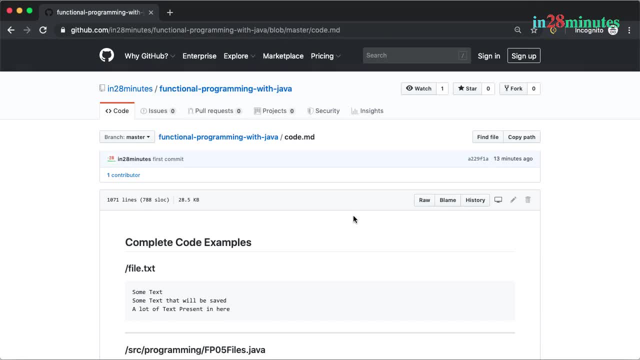 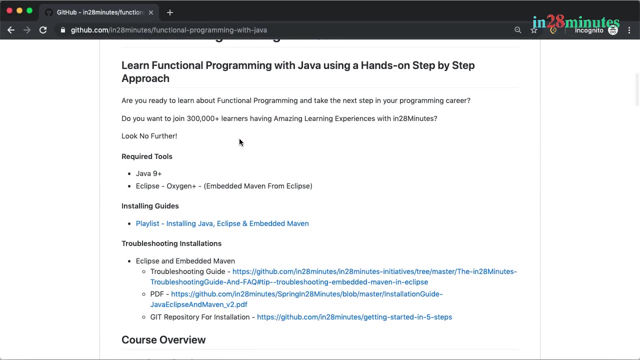 If you face any problems during the code, you can always refer to this file and find out what needs to be fixed. The exercises file contains the details of all the exercises and puzzles that we would solve during this course. If you scroll a little down, you would see an installation guide which would help you to install Java and Eclipse. 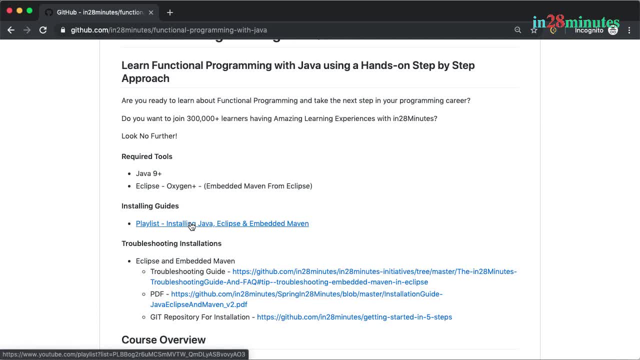 If you don't have Java or Eclipse installed, I recommend you to follow this guide and install the recommended version of Java and Eclipse. Any version of Java greater than Java 9 should be fine. We would recommend you to use as latest a version as possible. 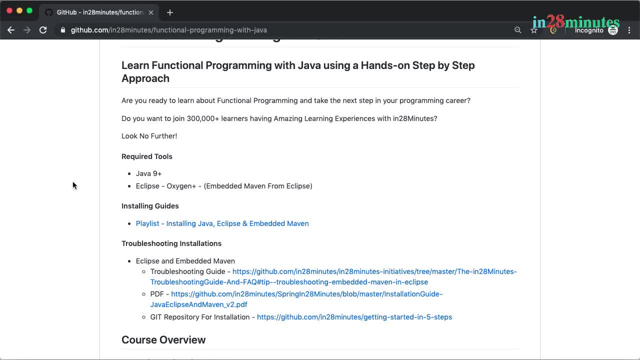 For example, Java 11 or 12.. And any of the latest versions of Eclipse should be cool. If you face any problems with installing the tools, we also have a troubleshooting guide present in here. Cool, Cool, So make sure that you bookmark the GitHub repository. 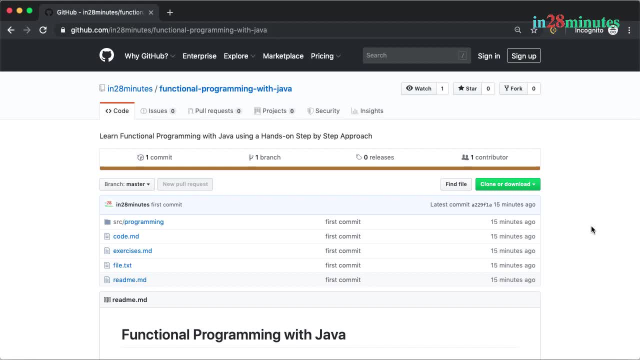 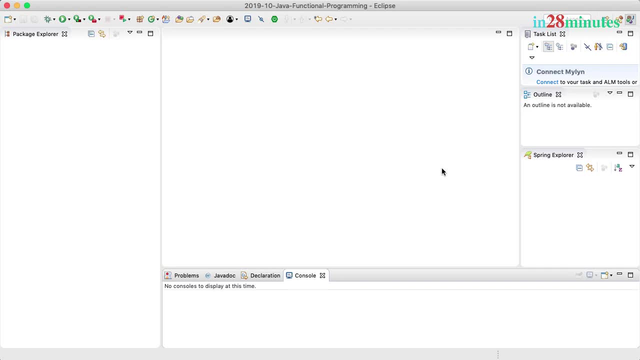 And make sure that you have Java and Eclipse installed, And I'll see you in the next step. Until then, bye-bye, Welcome back. Let's now jump right in. One of the first things that you need to understand is functional programming is a paradigm shift. 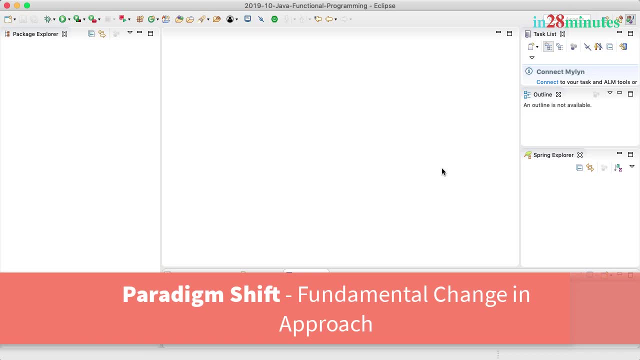 What do I mean by a paradigm shift? It means that you would need to change how you would think about problem solving To master functional programming, And we are here to help you make that transition. In this course, we'll take a step-by-step approach to introduce functional programming to you. 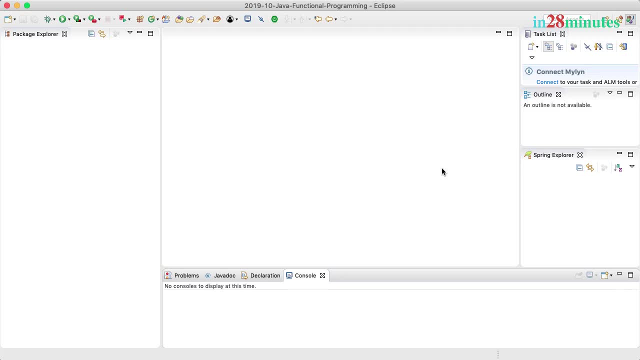 In this first section, we start with two key objectives. Number one is to help you understand how functional programming is different. Number two is to help you understand a few basic functional programming concepts. We'll talk about streams. We will talk about lambda expressions. 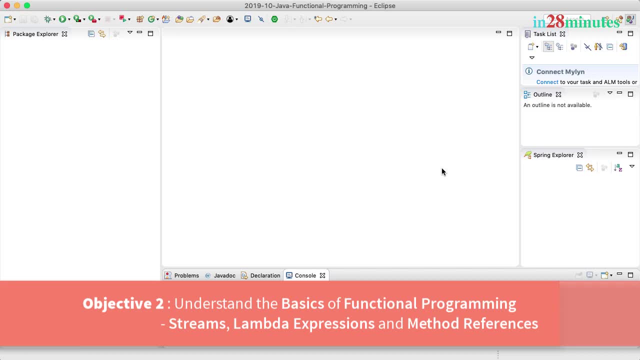 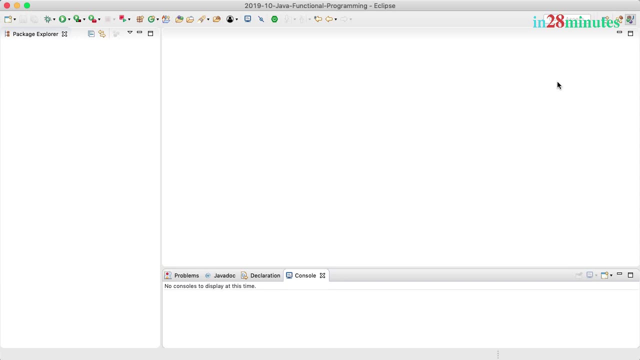 And we will talk about something called method references. As usual, we'll take a very, very hands-on approach towards learning functional programming. We'll write a few examples in traditional approach And look at how you can write similar code in functional programming. 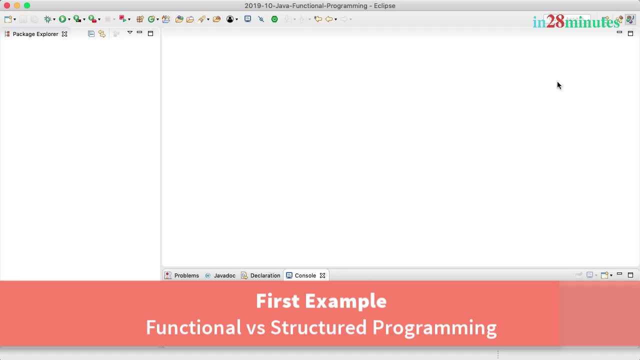 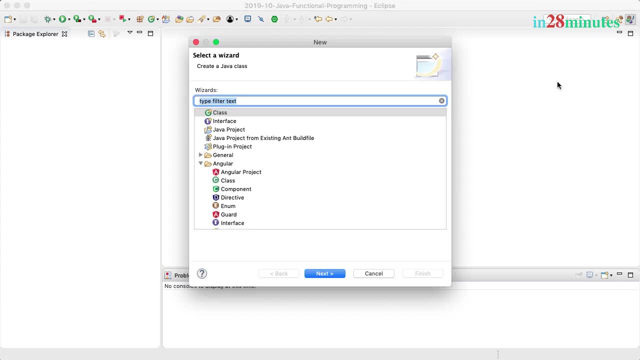 Let's quickly get started creating a new project and starting to write some code. I'm going to create a new project. I have Eclipse open. I have already chosen a workspace. I would want to create a new project, So let's go ahead and create a new Java project. 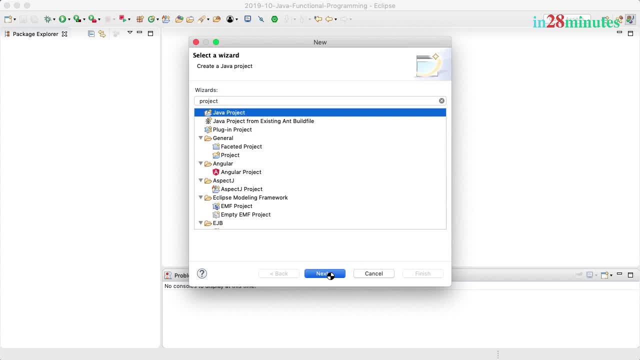 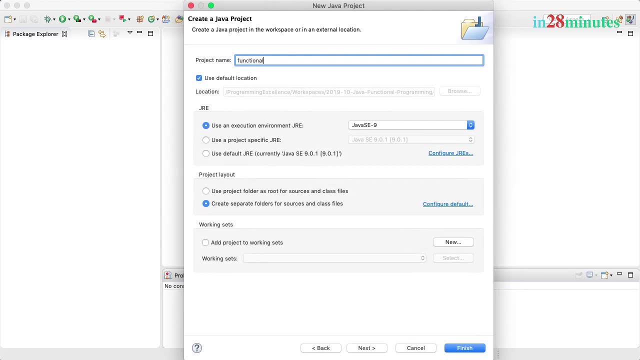 That's what you would want to create. File new Java project And let's give the project a name. I'll just call this functional programming with Java. As you can see, in here I'm using Java 9.. Any version of Java greater than 9.. 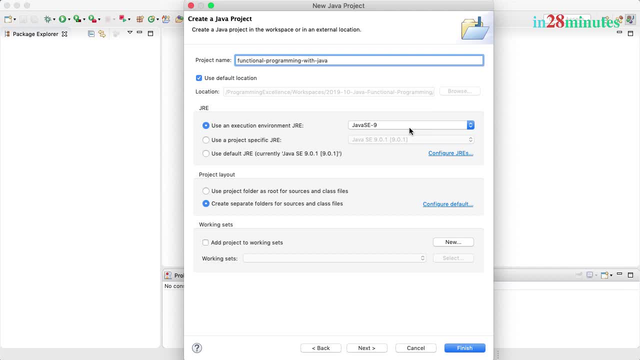 9 is cool, So Java 9,, 10,, 11, 12.. The code which we write in this course is compatible with all the versions. That's the only thing you would need to do, And after that you can say finish. 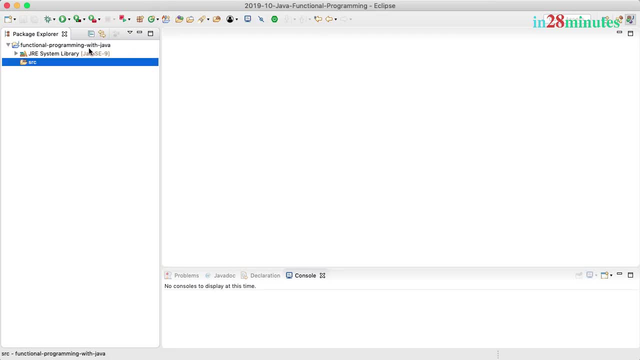 Now the project is created for us, We have a source folder where we can write our source code. Let's get started with creating our first example. The first problem that we would want to solve is: we would want to print a set of numbers. 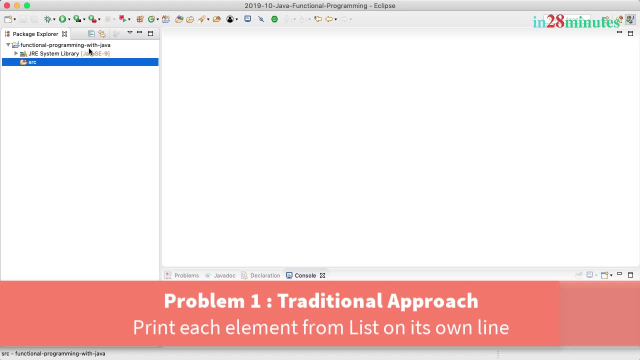 So we'll have a list of numbers, And we would want to actually print each element in that list one by one on a separate line. Now how do we do that in a traditional approach? Let's quickly look at it. I'll create a new Java class. 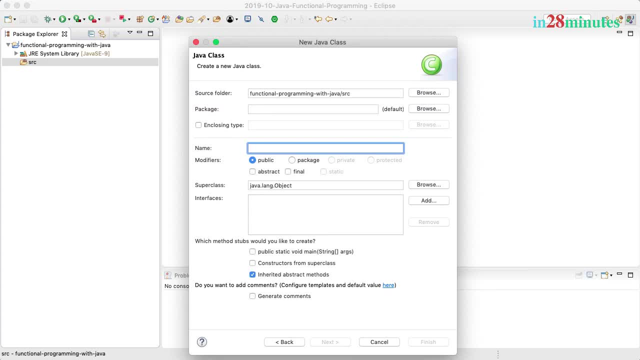 So I'll say new class And I would want to give it a name of FP01.. So we would use functional programming. 01 is where we are in right now And I'll call this structured, So FP. structured is the name of the class. 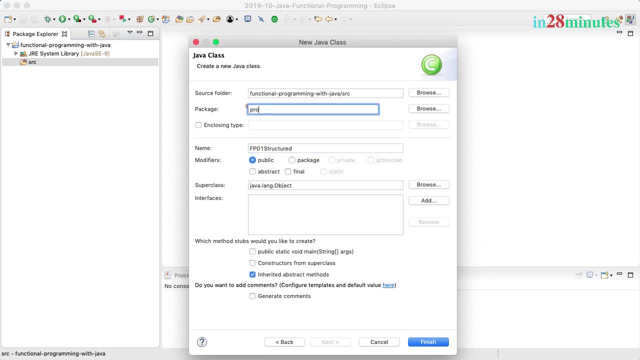 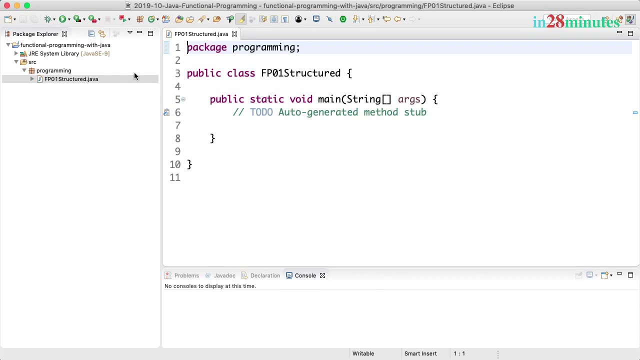 And the package name. I would give it as programming. Let's add in a main method And let's click finish. This would create the class for us with the main method, which is present in here, And over here I can write all the code that we would want. 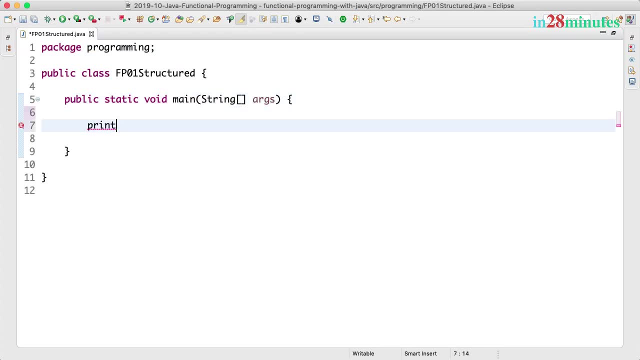 So what do we want to do? We would want to write a method to print all numbers in list. And which approach do we want to use? We want to use a structured approach, which is the traditional programming approach. Structured approach: What do we want to print? 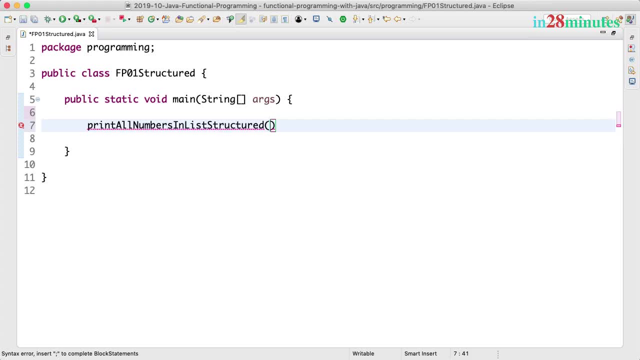 We want to print a list of numbers. How do we create a list of numbers? I can say listof, Let's enter a sequence of numbers. This can be random numbers. So let's enter 12,, 9,, 13,, 4,, 6,, 2, 4.. 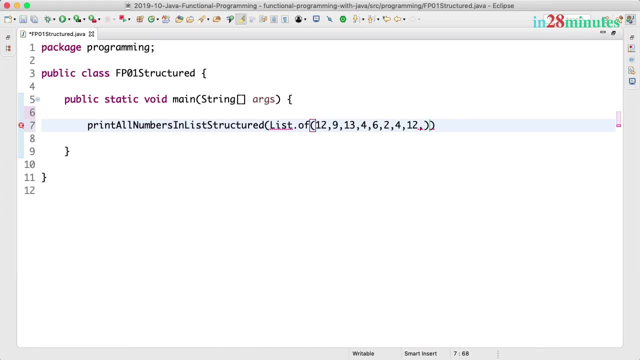 Let's have a few duplicates as well, So 12, 15.. Let's have a set of numbers in here. Now. it's first giving me a compilation: errors on the list. Why? Because I'm not really imported it in. 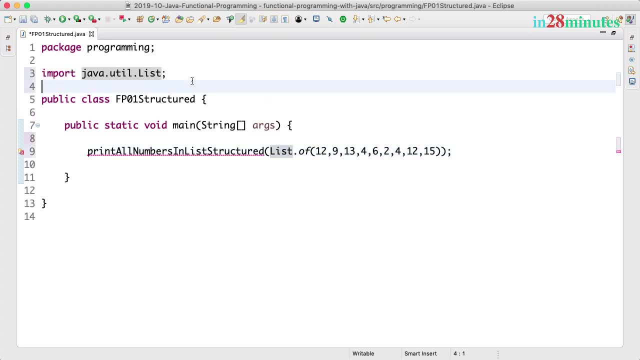 So I would want to use javautillist. So over here you can see that it's now imported in javautillist. I just needed to do control 1 or command 1 and take the option to import javautillist. Aha. 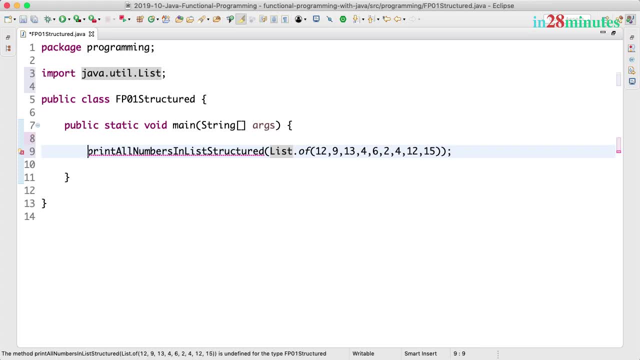 The method does not really exist, Right. So I can create the method right now: Control 1 or command 1.. And it says: create the method. Please do create the method for me. Cool, The method is now created for us. 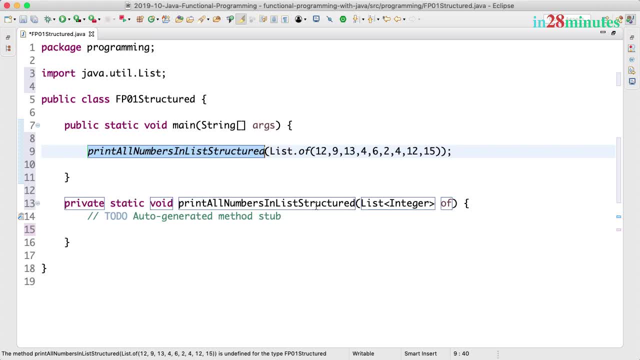 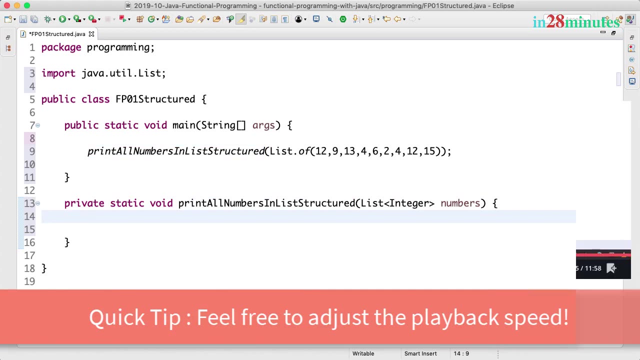 You can say it's private static void. Print all numbers in list structured And I'll want to give a name over here. I want to call this numbers And I'll remove this line. Control D, command D And over here. 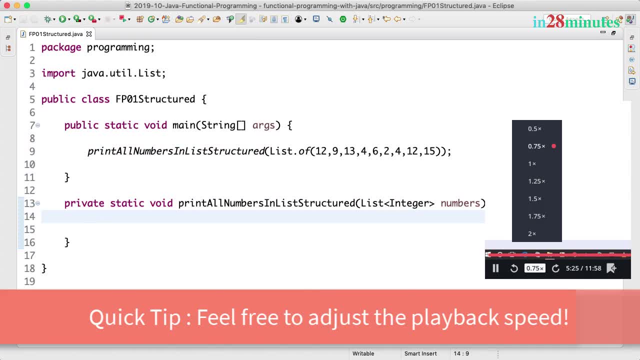 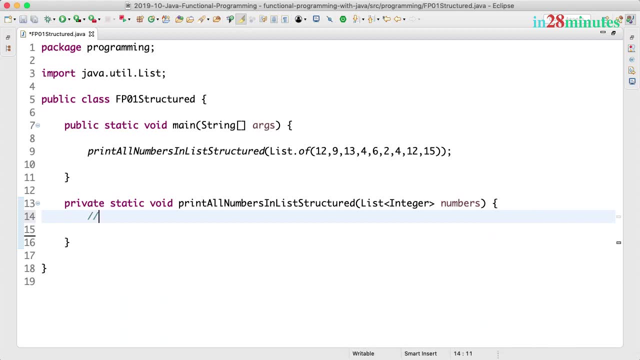 I'll print all the numbers in the list. Now you can write the program by yourself. How do you write it? The first thing that you need to think about is how to loop the numbers. That's this traditional approach, Right? So we would want to first figure out how do you loop all the numbers? 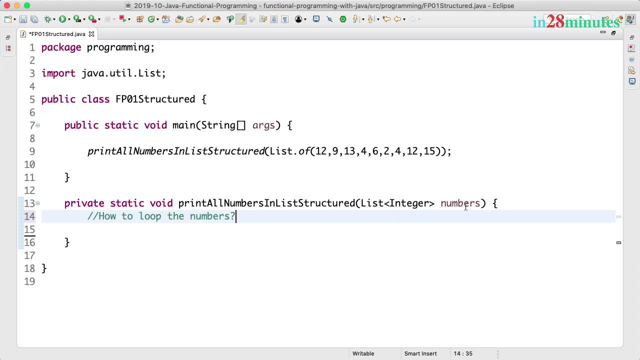 And once you decide how to loop, you can take each of the individual numbers and print it. So we'll first choose between: okay, should I use a traditional for loop Or should I go for enhanced for loop? Let's use the enhanced for loop. 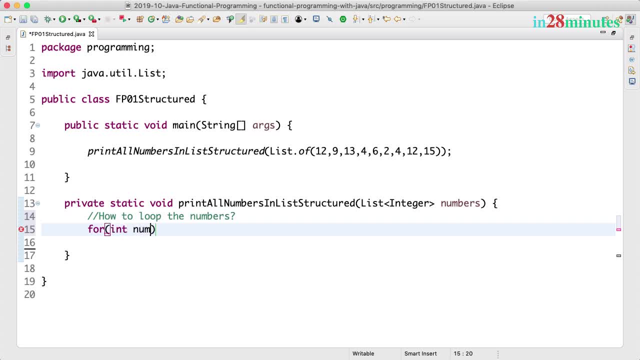 I'll say for int, number in numbers. What do you want to do? You would want to print them out. So sysout and number, Is that what you would want to do? So you would want to print all the numbers in list in a structured way. 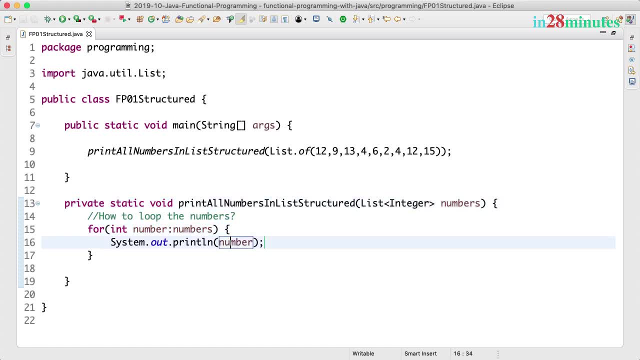 All that we needed to do was to loop The list of numbers And print them out. Let's run this and see what would happen. Right click, Run as Java application. Cool, You can see that everything is now printed out to the console. 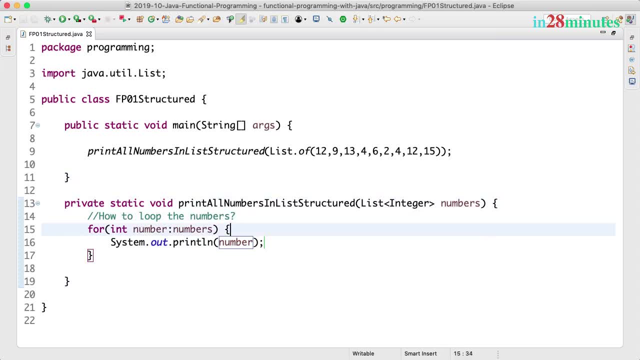 As you can see in here, in the traditional approach, whenever we would want to solve a problem, we focus on the how. The first thing we needed to do was: okay, I have a list of numbers. How do I loop around them? 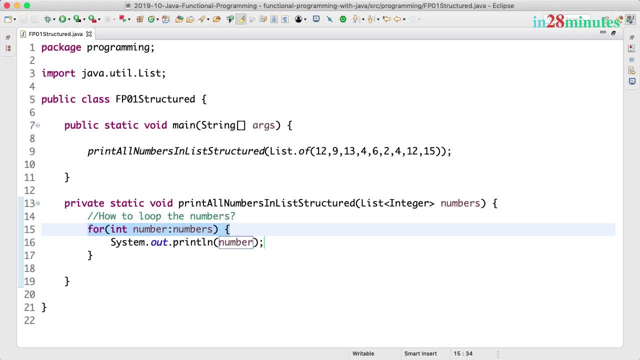 Okay, I'll use a for loop. That's the first thing that we did when we were talking about the structured approach. Now, how do we solve the same thing in a functional approach? I'll keep you guessing. Let's see that in the next step. 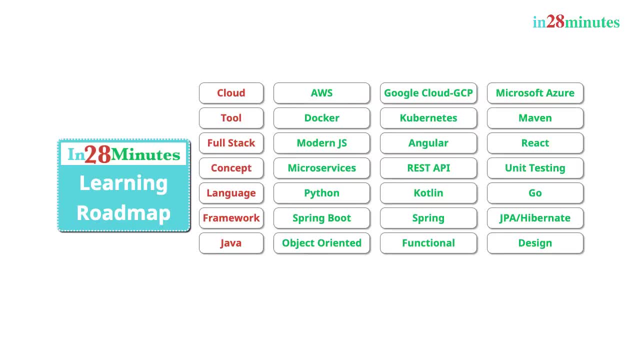 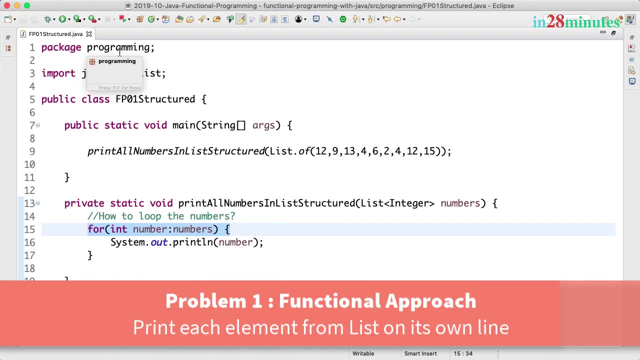 Until then, bye-bye, Welcome back. In the previous step, we solved this simple problem in a structured approach, And in this step we would want to focus on how to solve it in a functional approach. What I'll do is I'll copy this file and paste it down here. 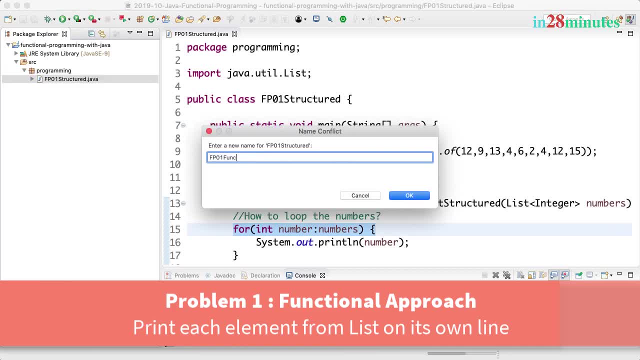 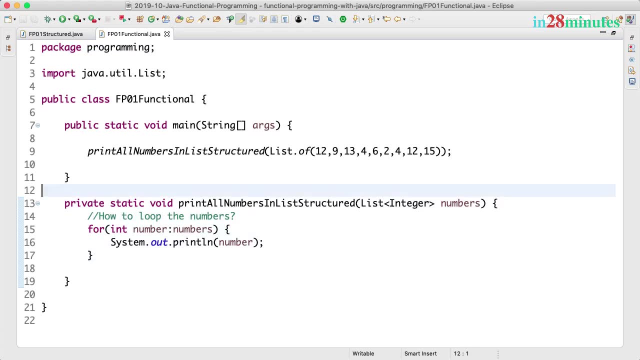 I'll rename it to fp01 functional. Let's open up fp01 functional And that's where we'll try and solve this problem. Let's start with renaming the method: Right-click refactor, rename, And I would want to rename this to print all numbers in list in a functional approach. 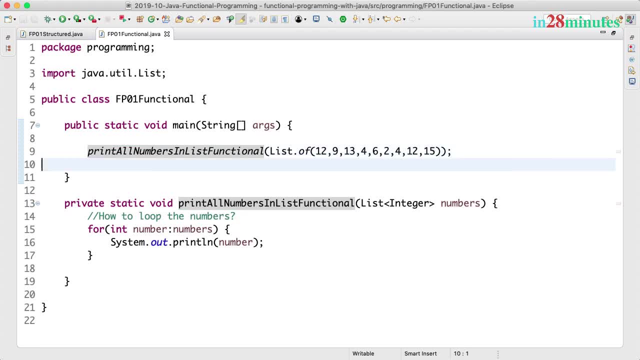 That's what we would want to do. We want to print all the numbers in a functional approach And we have a list of numbers passed in. Now, how do we do this in a functional approach? One of the important things to remember is: in the functional approach, we will focus on what to do. 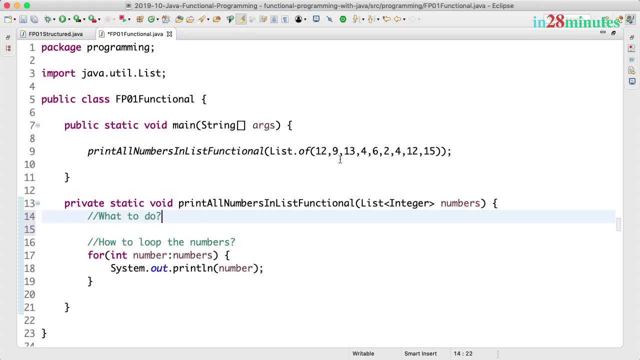 Before we can focus on what to do, what we would need to do is we would need to convert the list of numbers into a stream of numbers. What does that mean? You can see that the list of numbers is this: Let's convert this into a stream. 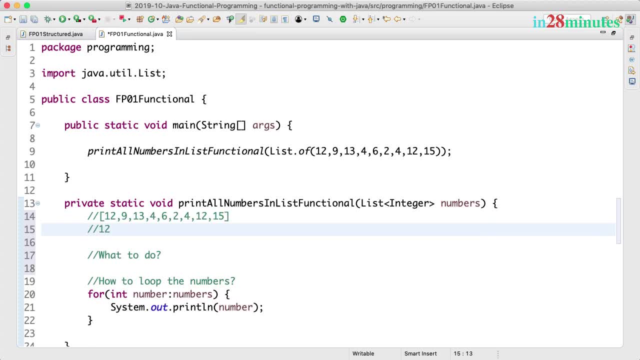 So I would want to convert it into a sequence of elements. I would want to first get 12, then get 9,, then get 13,, then get 4, and so on and so forth. So we would want to convert whatever we have into a stream of elements. 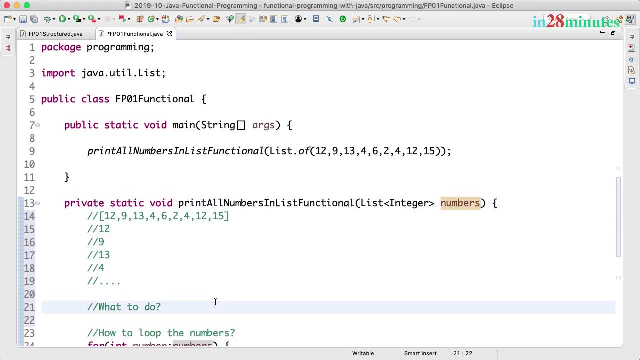 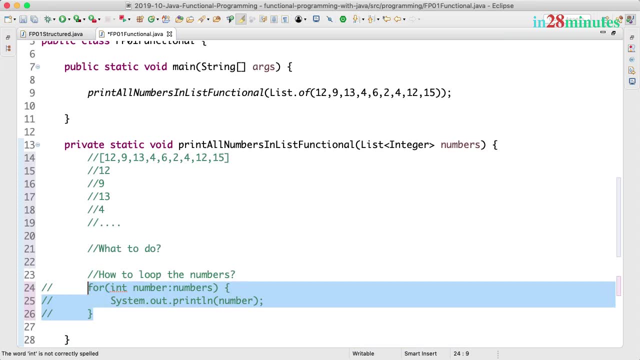 How do we convert a list into a stream? The way we can do that is by Let's comment out this piece of code: Control slash or command slash, and followed by control shift F or command shift F to format it. That's commented out. 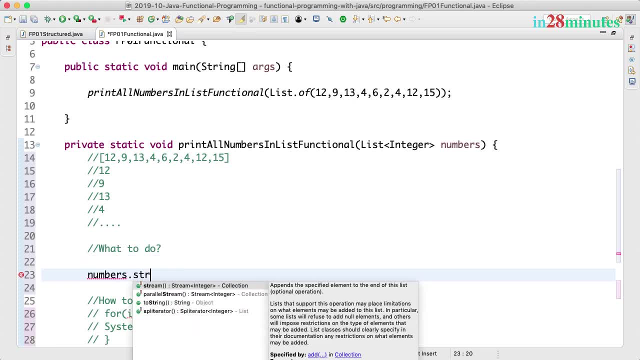 We want to create a stream for numbers, So numbers dot stream. As you can see in the Java doc it says: returns a sequential stream with this collection as its source. So we are taking a list and converting it into a stream of numbers. 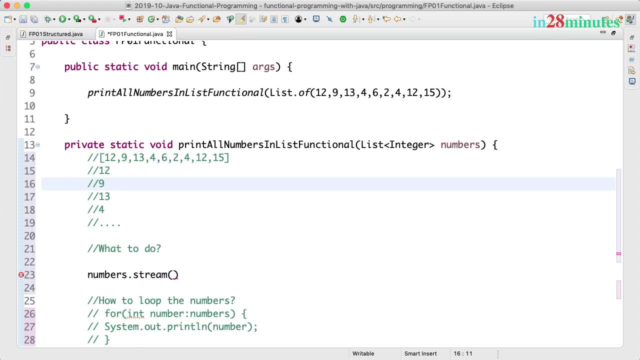 So we are converting it into individual numbers which come one after the other, A sequence of numbers: 12,, 9,, 13, 4.. Once I have a stream of numbers, what I can do is to specify what to do with each one of them. 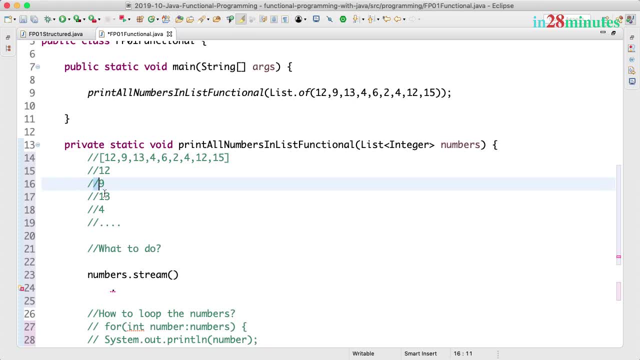 So when I get 12,, what needs to be done? When I get 9,, what needs to be done? What do we want to do with each one of them? We want to do a system. dot out, dot println number Right. 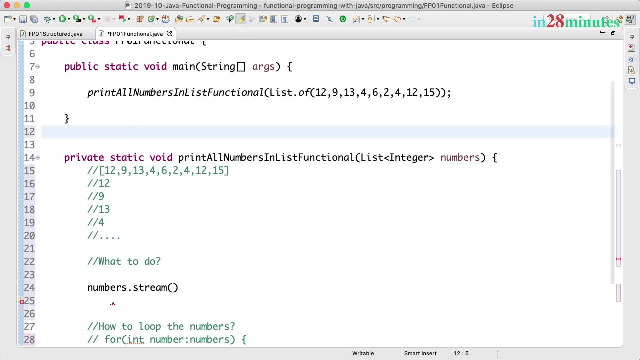 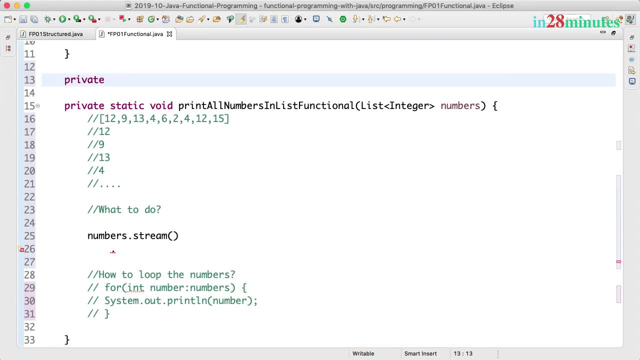 So what we'll do is we'll create a simple method which accepts a parameter And prints it out. So let's create a simple method in here. So I'll call this private static void, I'll just call this print And let's send in a int number to it. 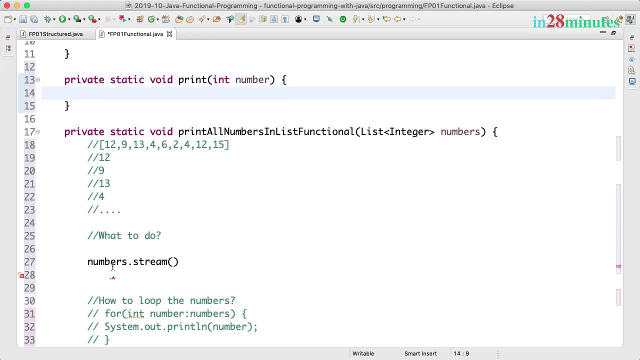 What this will do is it will just do a system out dot println number, So it just prints a single number, That's it, Nothing more, Nothing less. Now, what do we want to do over here? Numbers: dot stream For each number. 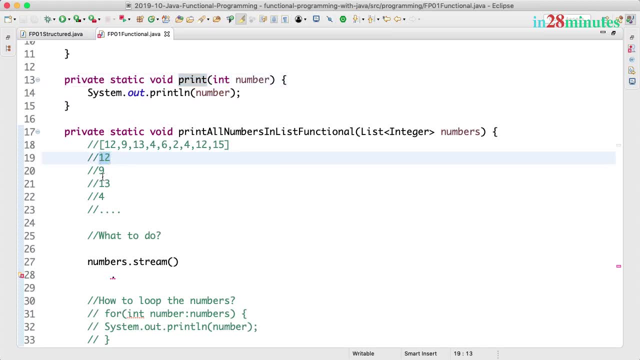 For each of these numbers: For 12., For 9., For 13., For 4.. We would want to call the print method. How do we call the print method from here For each of the numbers? The way we can do that is by saying: for each. 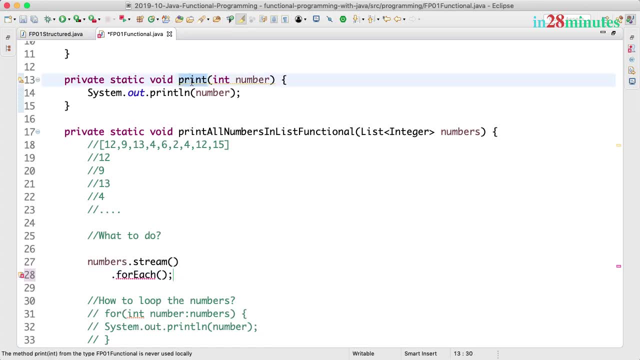 And you can define- I would want to call the print method Now over here- typically what we would do. we'll say: print of 5.. Right, So typically what would happen? This code would be immediately executed. We don't want the method to be immediately called. 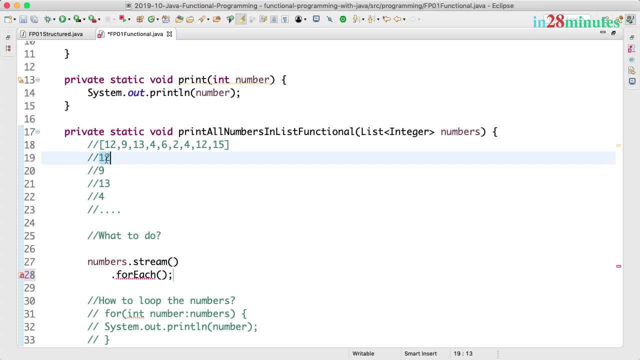 What we would want to do is to define what needs to be done. We need to define the behavior when we get a number of 12.. To define the behavior, we use something called a method reference. How do you put a method reference in? 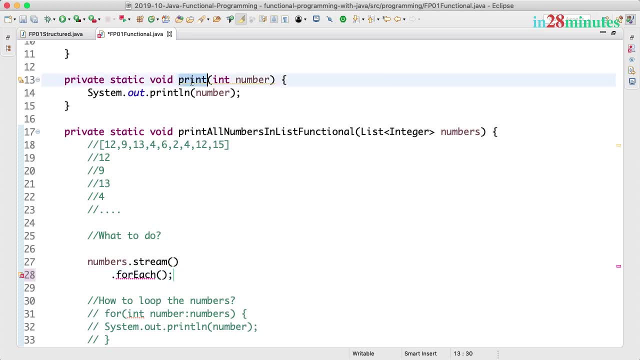 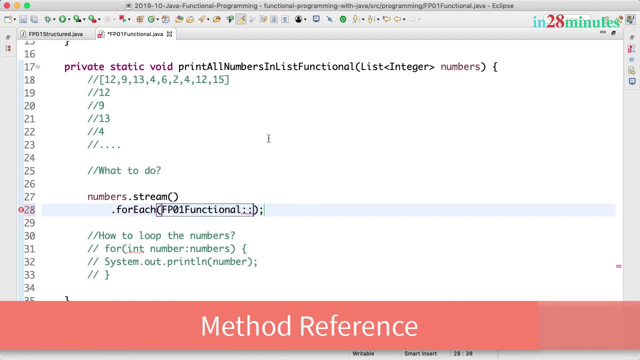 What we want to do is for each element, we would want to call this print method. How do we say that? The way we can say that is by using the name of the class colon, colon followed by the name of the method. So you can see that this is a static method. 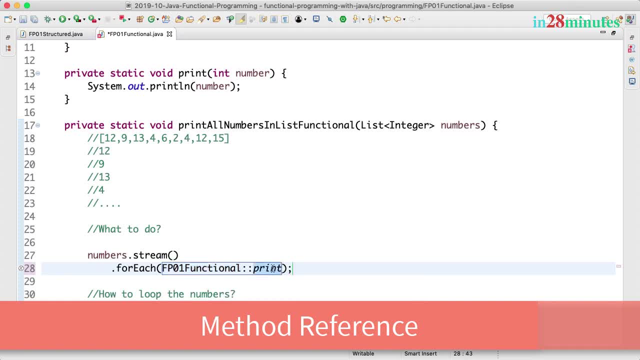 And I'm using the class name colon. colon, the name of the static method, And what I'm telling it is: hey, take the numbers, convert it into a stream And for each element: for 12,, do a print. For 9,, do a print. 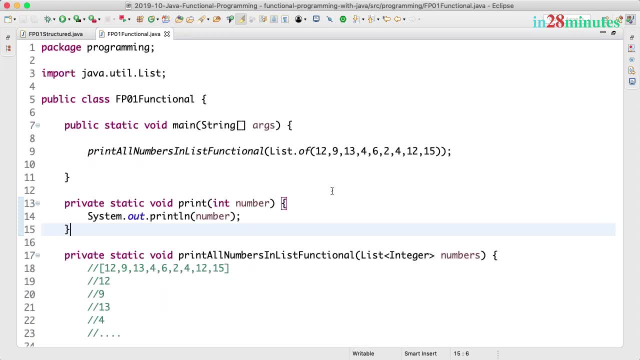 That's basically what we are specifying in here. Now I think we have got almost everything covered, So let's do right-click, run as Java application. Aha, The output does not really change. You can see that everything is being printed out in a sequence. 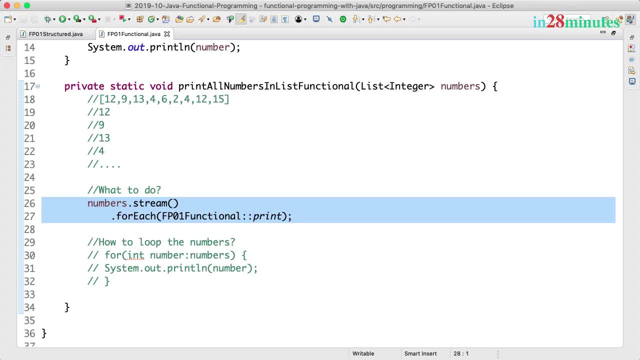 Let's end this step by reviewing quickly what's happening with this code. What we are doing is we are converting the numbers list into a stream. So instead of getting a list like this, what we'll get is a stream of elements like this: 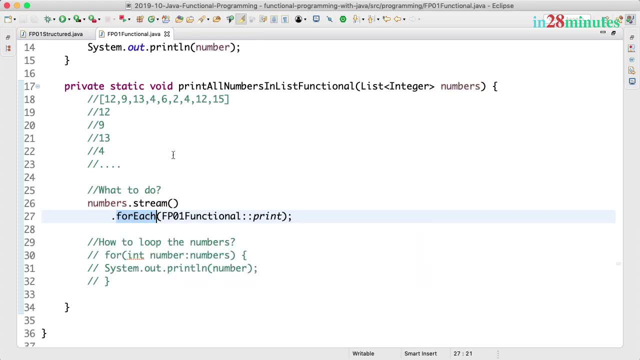 And what we are specifying is for each of these elements which are coming out. what we would want to do is to call the print method which is present in the current class And the syntax which we are using in Java. what we are saying in here is colon colon. 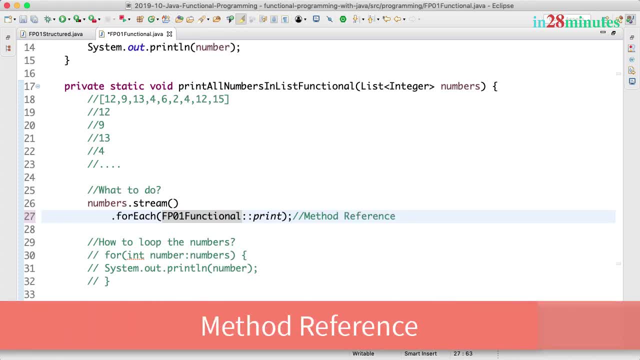 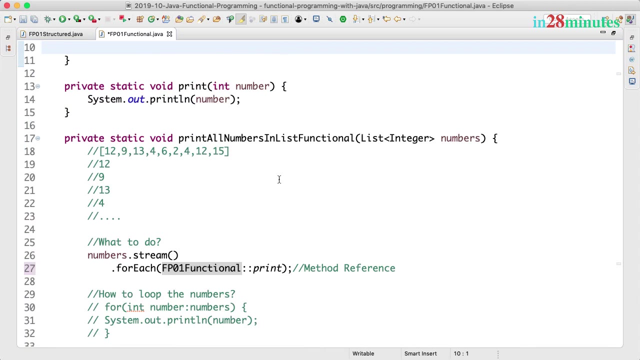 This is the syntax of something called a method reference. What we are saying in here is: for each element, this method needs to be called. So for each of the numbers coming up, what would happen is this print method would get executed, And that's how we were seeing all the elements that are printed. 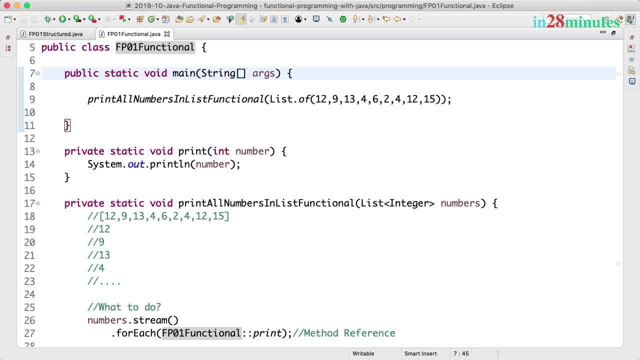 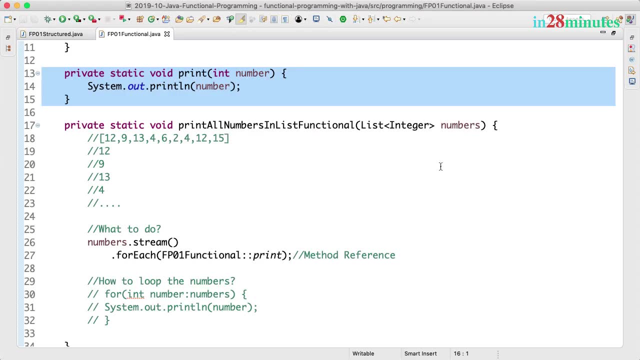 I'm sure there are a lot of questions about this specific approach. Hold on to them and I'll see you in the next step. Welcome back. In the last two steps we implemented a simple problem in a structured approach and the functional approach. 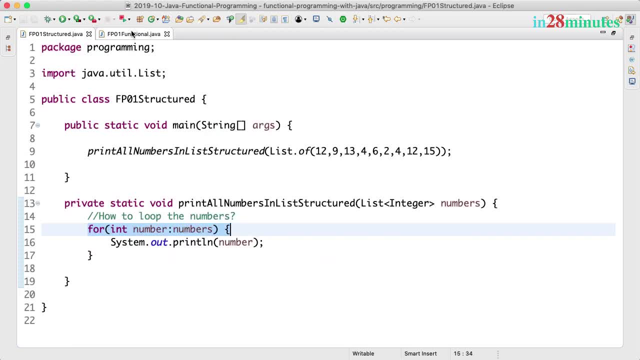 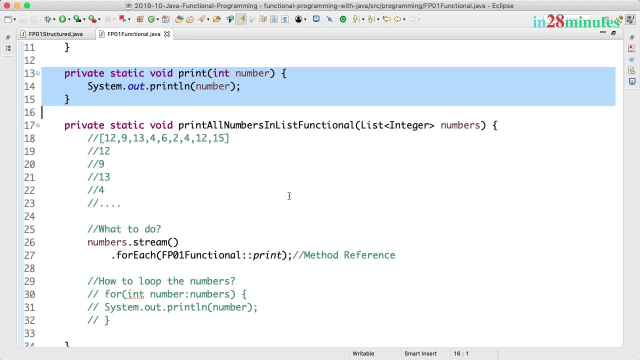 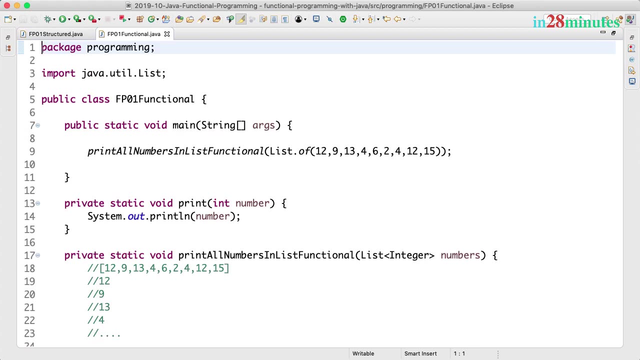 And you might be thinking now that the functional approach is much more complex than the structured approach, And that's true. with the implementation that we have right now, Let's see what we can do to simplify the implementation. So let's first remove all this stuff that we have in here. 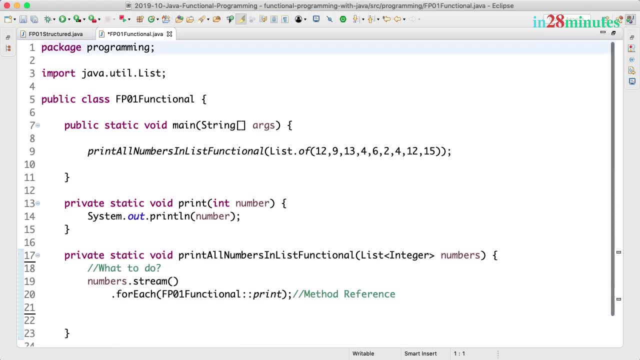 So let's actually remove the earlier code that we have inside the functional method. I'm using control D or command D to remove a line, And now let's see the need for this specific print method. What we are doing in here is we would want to call fp functional colon, colon print. 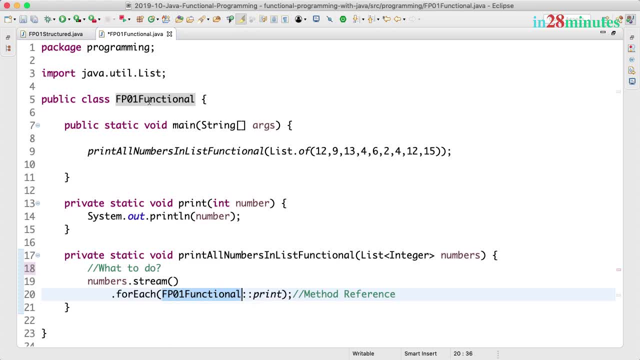 So we would want to call a static method in this specific class And what happens is, for each element in this stream, this static method is called with that element. So this stream contains a list of numbers, So first 12 is sent to this method. 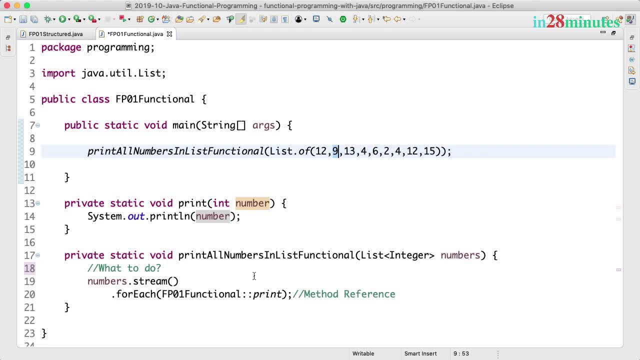 Next 9 is sent to this method. Next 13 is sent to this method, And we saw everything is printed out to the console. That's cool. Now, instead of doing this, you can actually replace this piece of code by directly specifying system dot out in here. 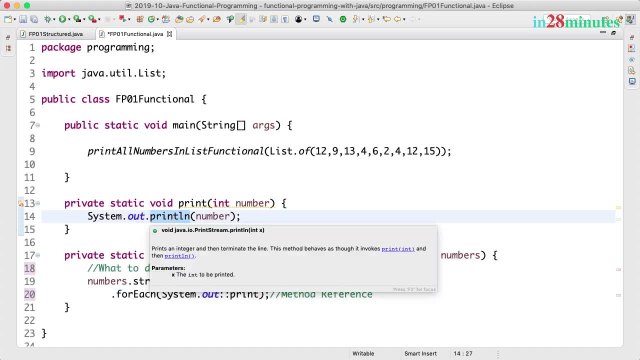 So system dot out? And what is the static method println? So system dot out contains a static method called println, And that's an easier way of doing it. Instead of creating a new method called print, what we can do is directly call system dot out, colon, colon, println. 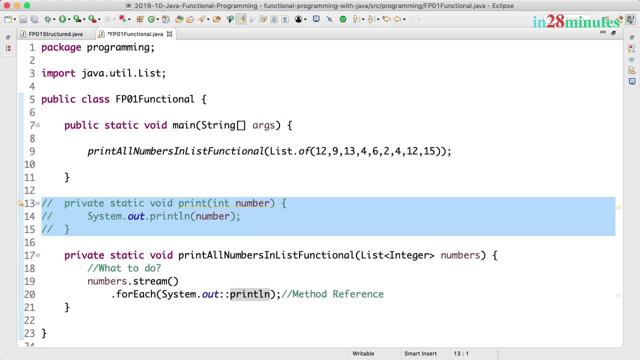 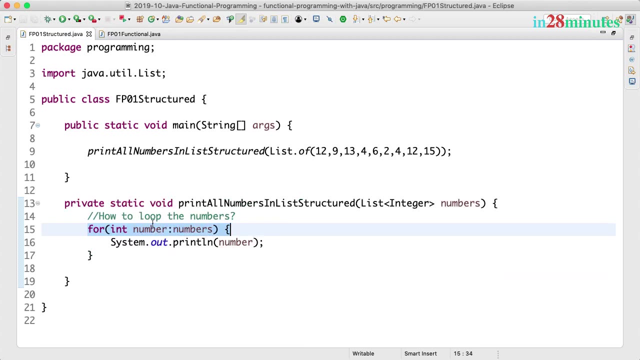 And now this method is no longer needed. So let's comment it out. Now. you can see that this piece of code is a little more simpler than the structured approach. Why do I call it simpler? Because in the structured approach, we had to focus on how to loop the numbers and then print them. 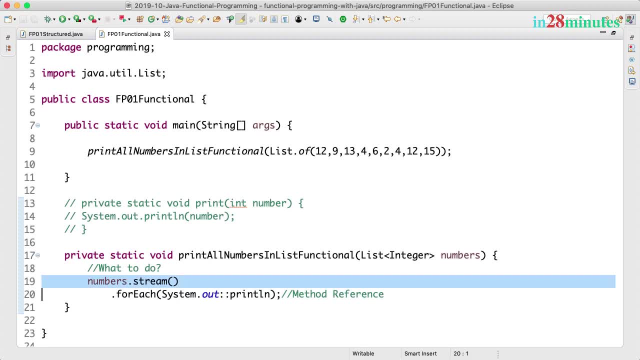 In the functional approach, on the other hand, we get a list of elements and we define what to do with each one of them. So all that we needed to do is to say for each element in this stream: do this. Now let's try and make the example that we have a little bit more complex. 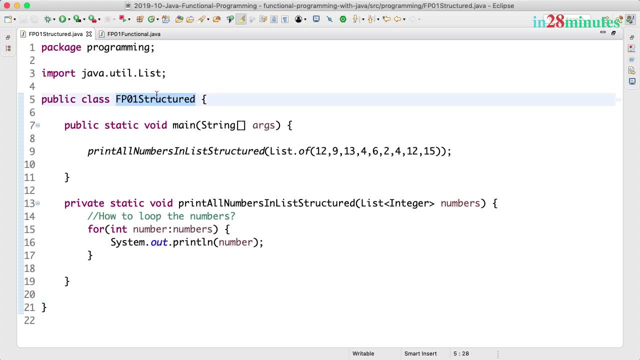 What I want to do is: I would want to go to the FP structured class And what I would want to do is to print only the even numbers. I don't want to print all the numbers in the list, but I only want to print the even numbers in the list. 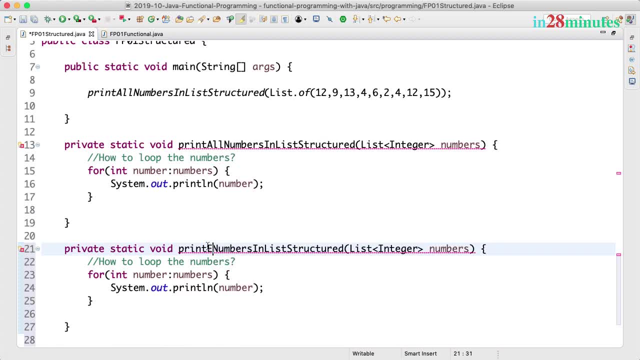 So instead of saying print all numbers in the list, I only want to say print even numbers in the list structured. How do we change this code to print even numbers in the list? Think about it Typically. what we would do is we would add the logic in here. 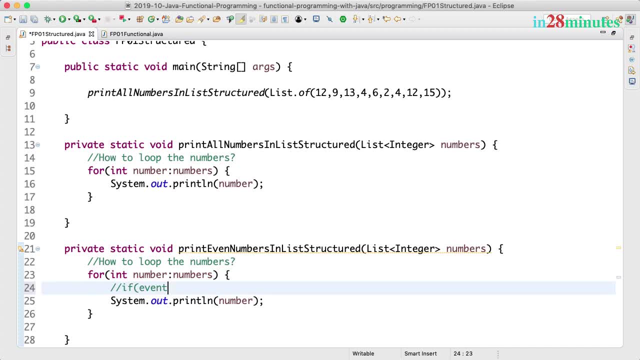 So we'll say: if this is even only, then print the number out. So let's do that. So if even, how can I check that the number is? even If number we can divide by 2.. So number mod 2 is equal to is equal to 0.. 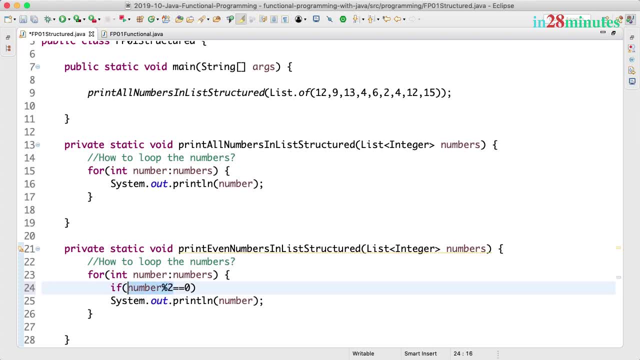 So we are dividing by 2 and checking the remainder. So number mod 2 divides the number by 2. And check the remainder. If it's 0,, then what we want to do is we would want to print the number out. 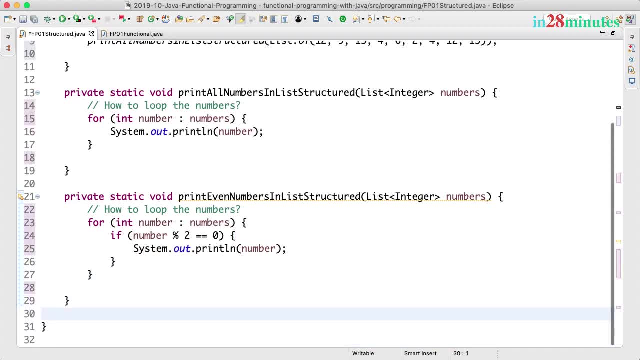 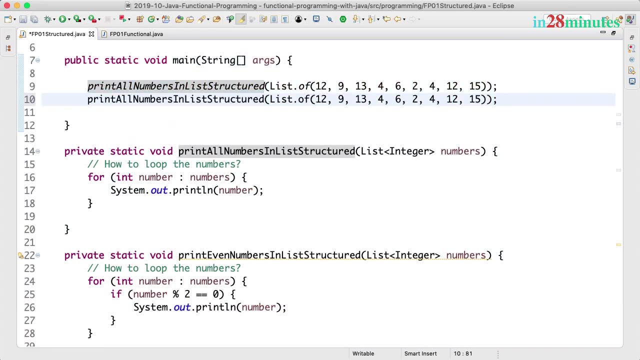 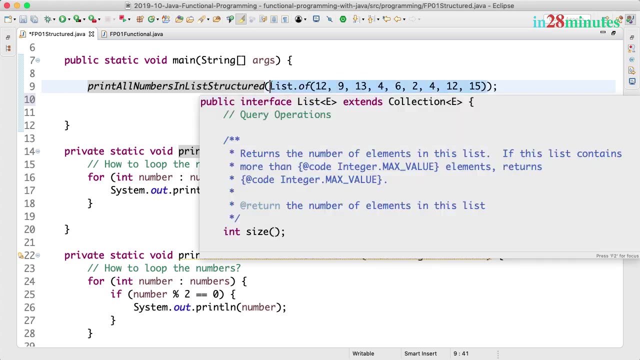 So let's format this out And now, if I call this so, print even numbers in list structured. I can copy and paste this in, but then I would be repeating the list. I don't really want to do that. So what we'll do is let's extract this list to a local variable. 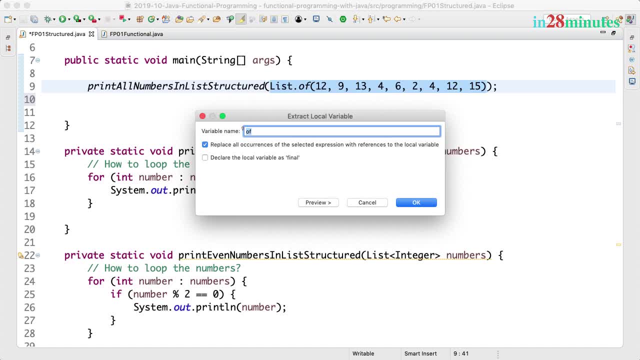 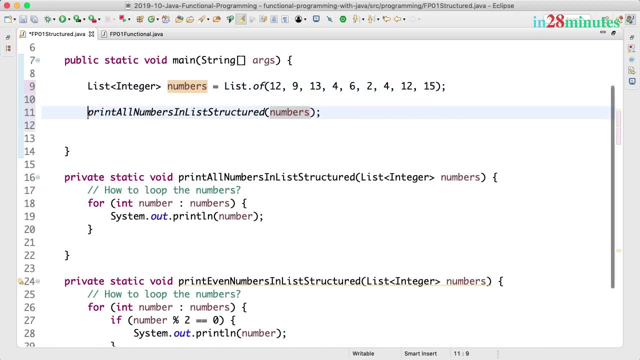 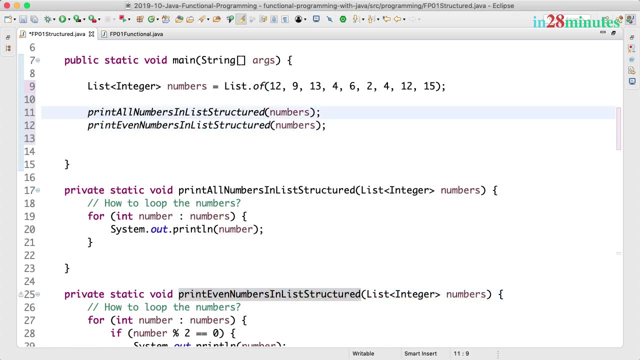 So, like quickly factor extract to a local variable, and the local variable that I would want to create Is numbers, And over here what we want to do is we would want to print all the even numbers in the list, Right? So that's basically what we want to do. 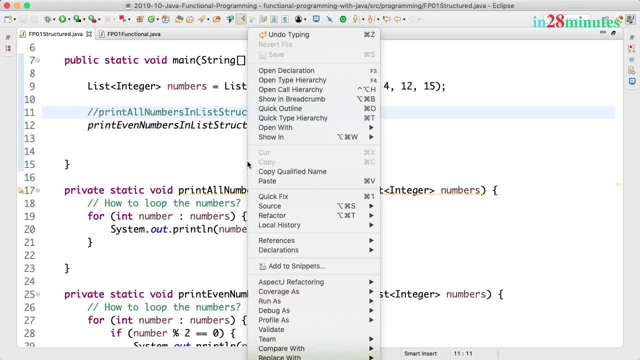 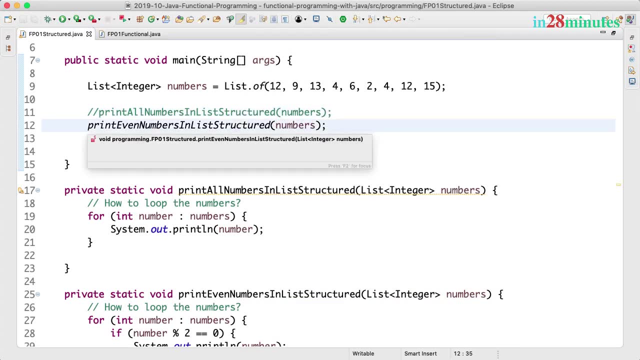 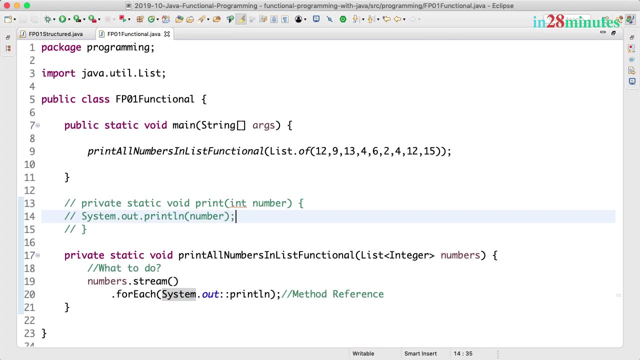 So we are using the structured approach and let's run as Java application. What would happen? Cool, Only the even numbers are getting printed. Now how do we do the same thing in a functional approach? How do I do that In a FP zero one functional class? 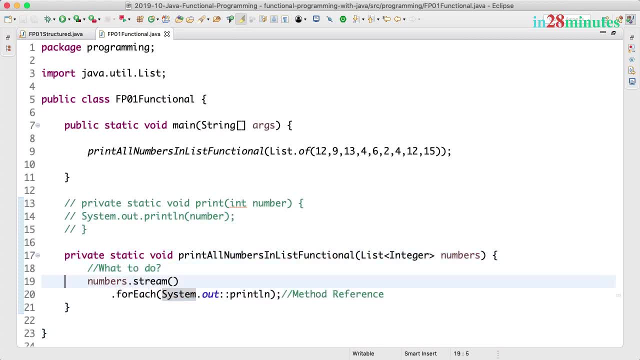 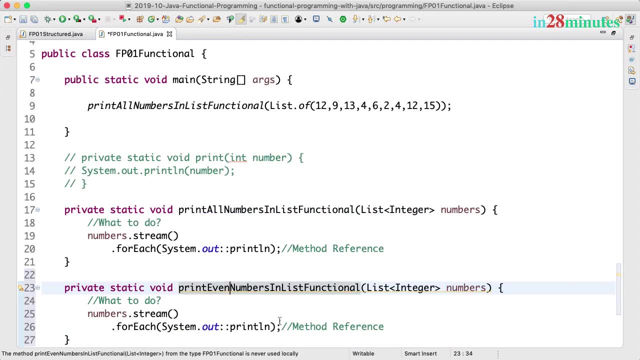 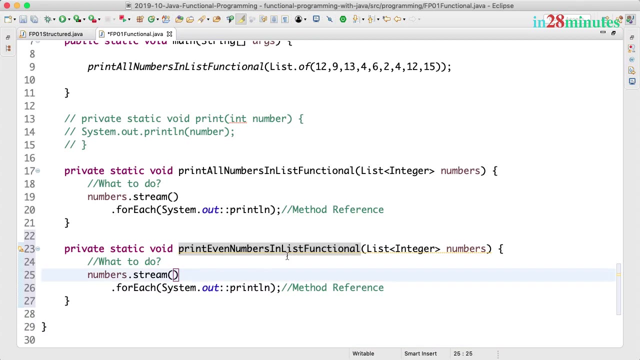 Let's see how to do that right now, So I'll copy the existing method. as usual, I'll call this print Even numbers in list functional And over here what we want to do is we would want to only look at the numbers which are even. 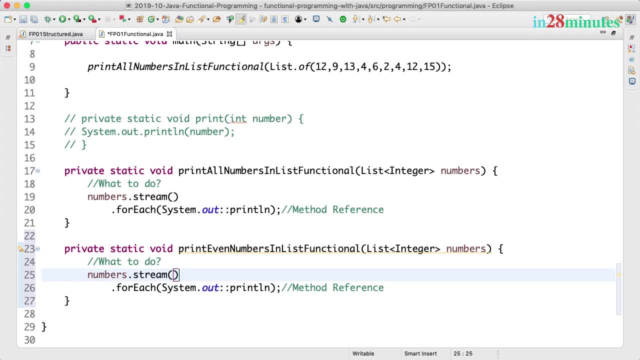 So how do I add additional logic in here? I can add a filter in here. I'll say: Only allow even numbers. How can I add a filter? The way I can do that is by saying dot filter. Now how do I decide if something is even? 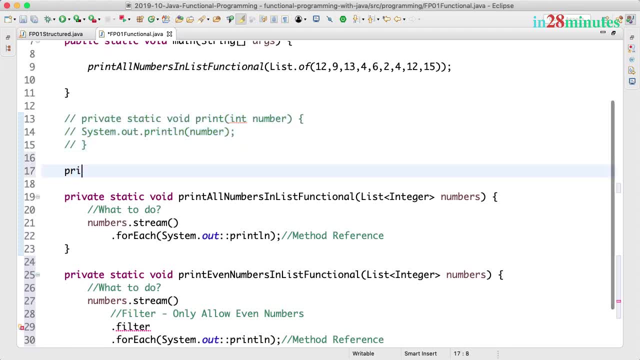 Let's create a static method for it. for now I'll call this private static. This should return whether it's even or not. So I'll say Boolean Private static. Boolean is even And let's pass a number to it, So int number. 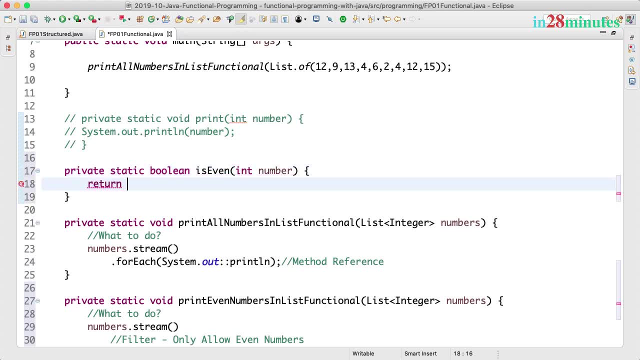 And this would return. What does it return? Number mod two is equal to is equal to zero. This is simple logic, right? All that it does is it divides the number by two, checks the remainder And if the remainder is zero, it returns true back. 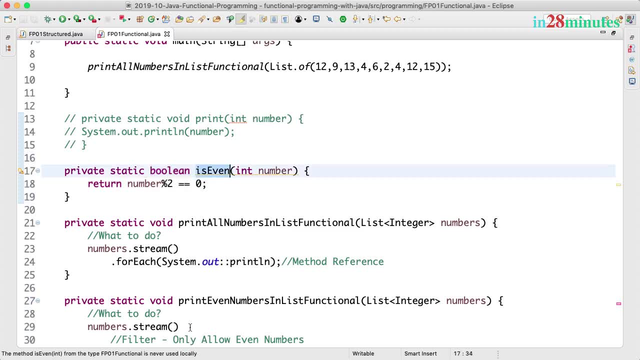 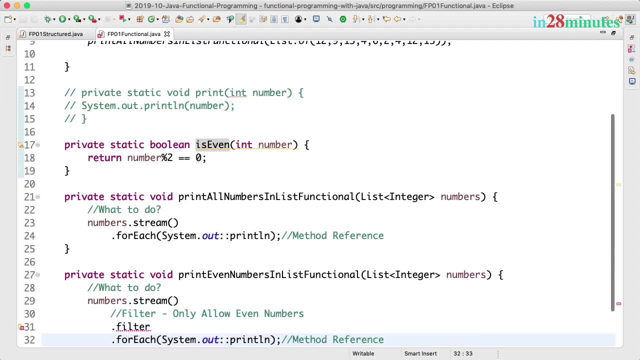 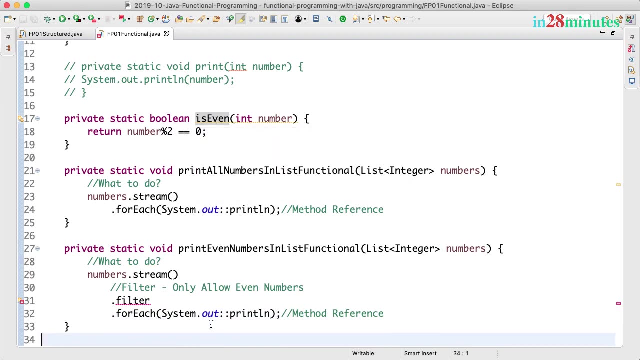 Otherwise it returns a false back. What do you want to do is we would want to call this method on each of these numbers And only if it is true, We would want to print the number. So you'd want to do a for each, only for the numbers where is even is written in true. 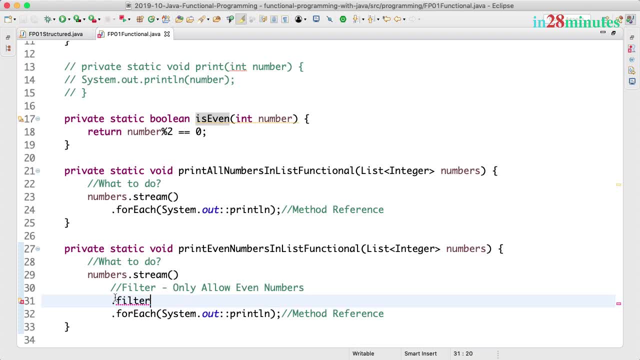 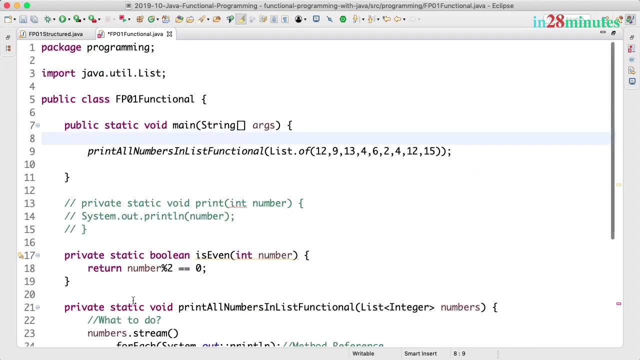 How do we do that? in the functional approach, The way we can do that is by creating a filter. So I said dot filter And over here I can say is even, And because this is a static method, the way we can define that is by using a method reference. 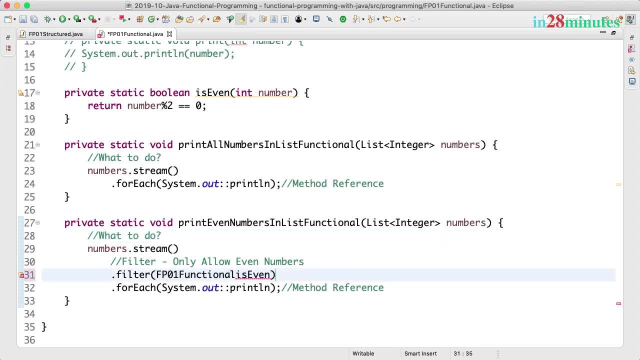 FP01- functional colon- colon is even. The important thing in the method reference is that we are not really calling it. We are not really calling it. We are just saying: okay, this is the method to be called. We are declaring that this is the method to be called on each of the numbers. 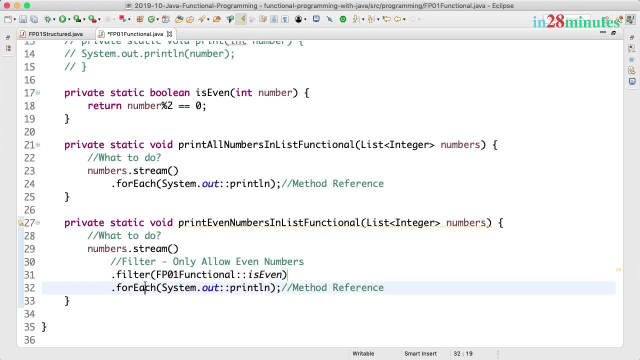 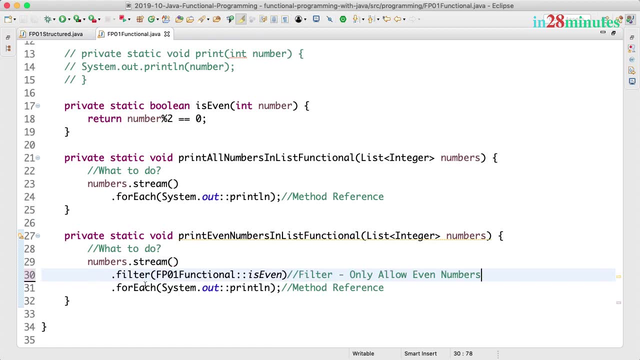 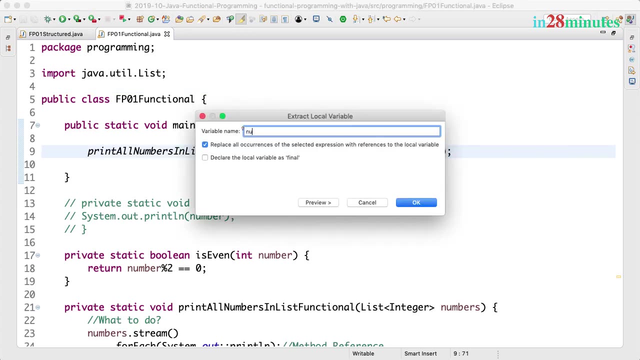 And if it returns true back, only then go to the next line of code. So let's move this comment out down to the side And let's now execute this. Let's quickly create a local variable for this list as well. Numbers: 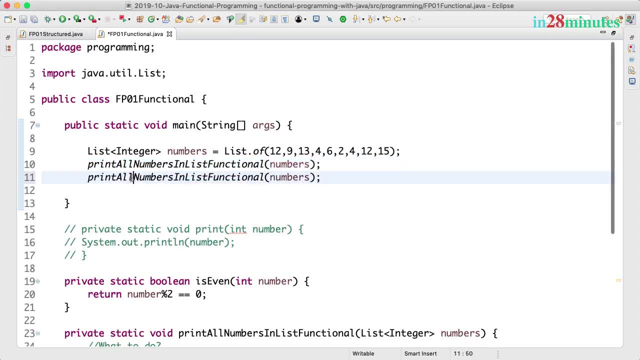 And what we want to do is copy this, And we would want to print even numbers in the list. Let's comment this out. Let's quickly run this and see what would happen. Do we get only even numbers? Yup, That's cool. 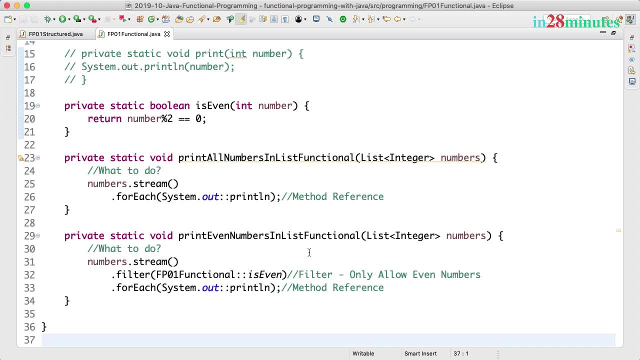 Now we saw that we were able to print all the even numbers in the list. Once again, you can see the fact that once we have a stream of numbers, all that we needed to do was add a check. So, for each number, do this check. 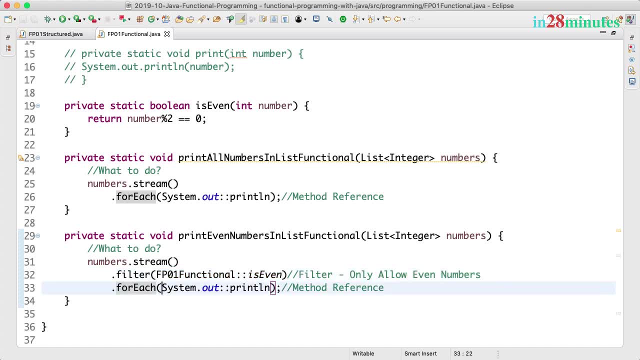 If that check is true, then you can actually go ahead and print the number out. Now again, you might be thinking that this method is a little bit more complex than the structured approach because we needed to use a method called ease. even How would it be if I can actually directly define? 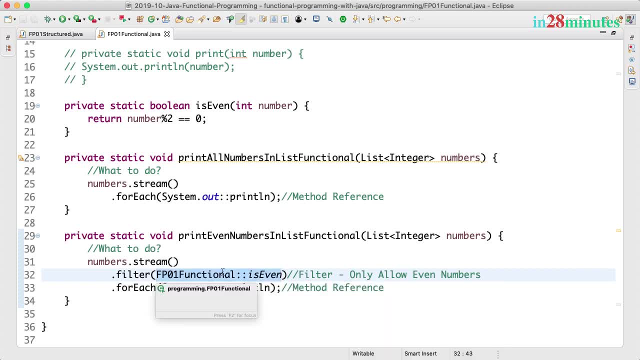 the entire ease even method in here, Instead of actually creating a separate method, having a return value, having the parameters defined, having the body, having the return and all that- can we do it in a simpler way and directly define the method in here? 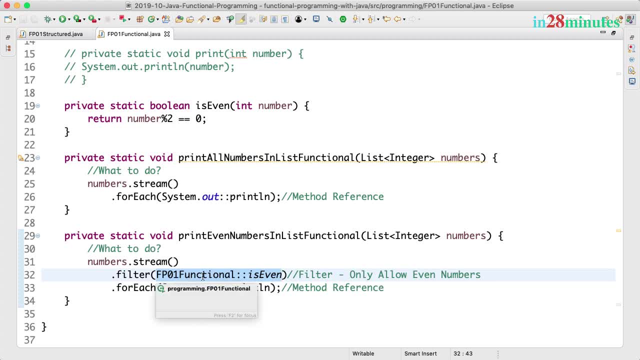 Let's look at that in the subsequent step. Until then, bye-bye, Welcome back. In the previous step we solved the problem for printing even numbers in a functional approach. However, we needed to create a separate method: ease even. 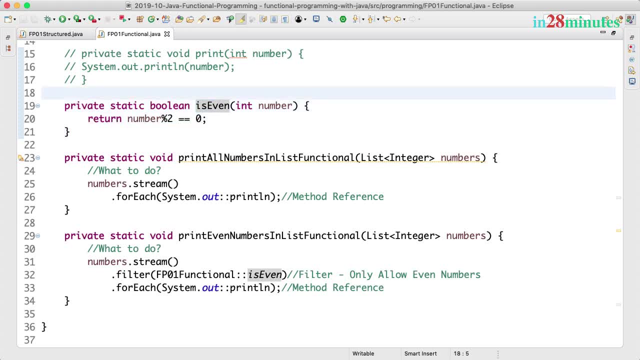 We saw that the logic for this method is very, very simple and we had to do a lot of ceremony, We had to add in a lot of detail to define the method and call it from here. Is there a simpler way of doing it? 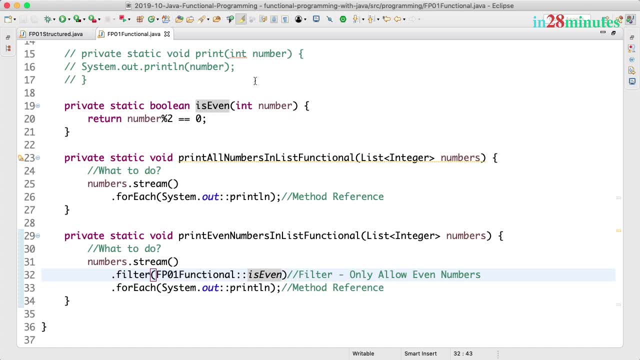 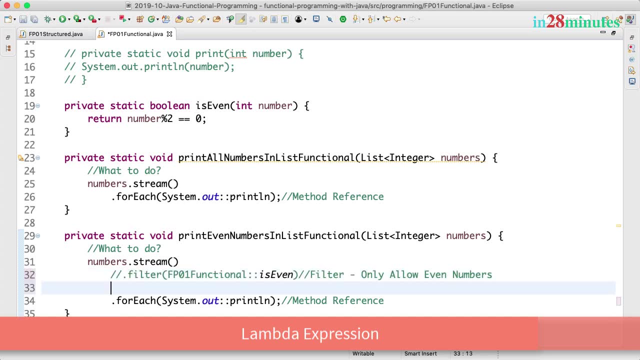 Let's look at it right now. The simpler way of defining this specific thing is called a lambda expression. What I'll do is I'll comment this and I'll say: dot filter Over here. what we want to do is we want to define a lambda expression. 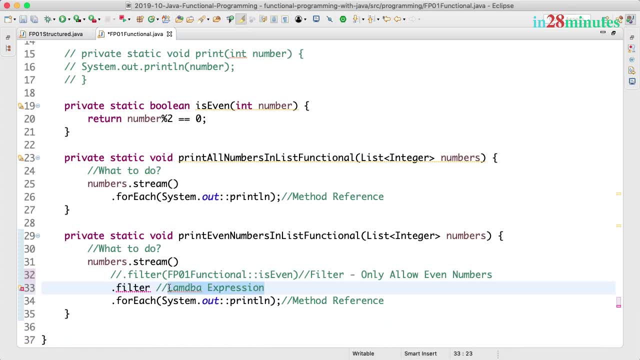 What is a lambda expression? A lambda expression is nothing but a simpler way of defining another method. Lambda expression is nothing but a method Very, very simple. However, in the lambda expression, you would use a simpler syntax for creating this method. 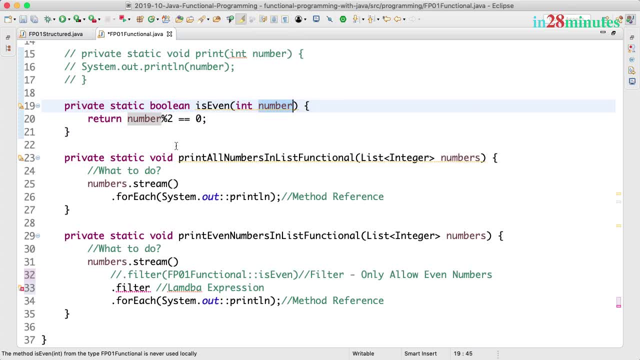 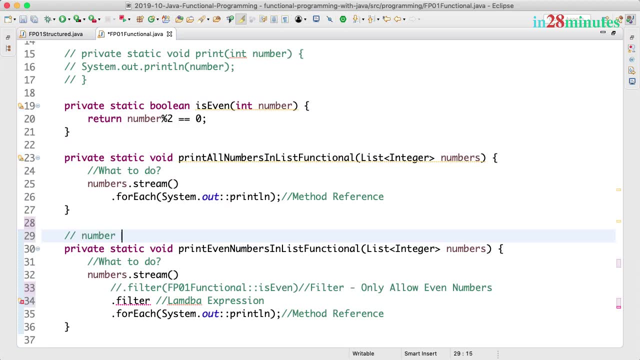 What does this method accept as a parameter? Let's start with that. This method accepts number as the parameter. What we want to do is we want to take number as the parameter and we would want to check. What do we want to check? 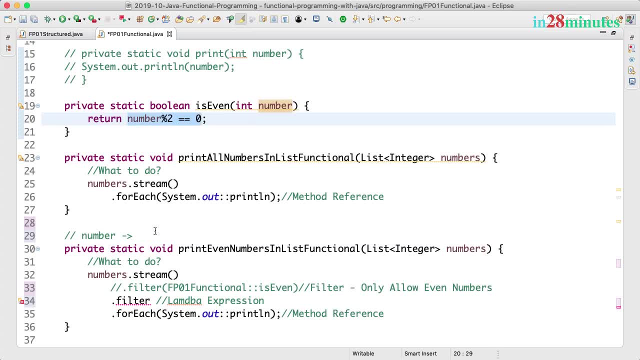 We would want to check if number mod 2 is equal to 0.. We would want to take a number and we would want to check if number mod 2 is equal to 0, and return it back. This is something of a special kind of a syntax. 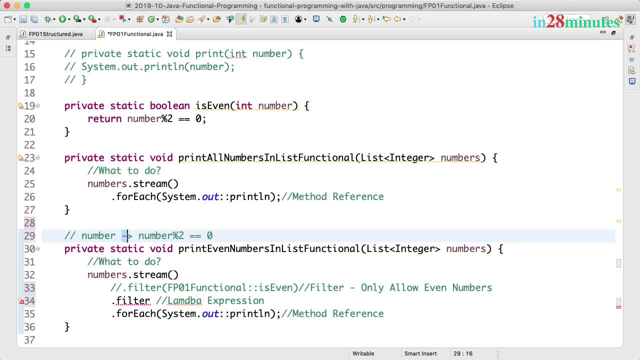 related to lambda expression. It's hyphen followed by greater than symbol. This is almost like an arrow symbol. What we are saying in here is: take the number in. Take the number and check if number mod 2 is equal to 0,. 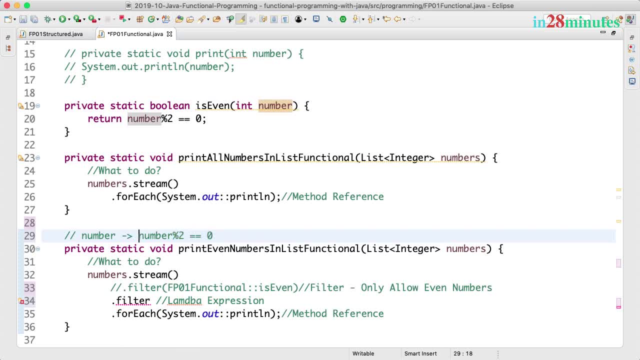 and return it back By default. in lambda expressions, if you just have one statement present, it would return that value back. What would happen in here? It takes the number and returns the value of number. mod 2 is equal to 0. 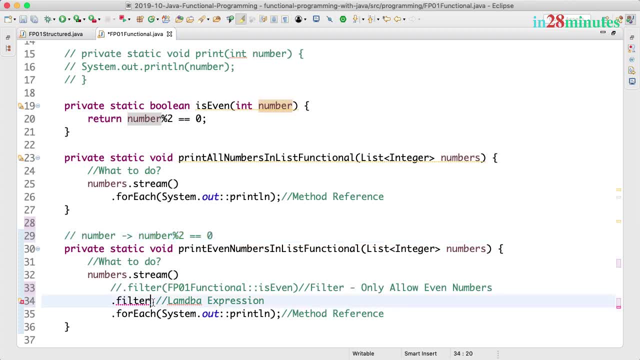 How do I use it in our code? I just need to copy this and put it in between parentheses of filter. What we are defining in here is saying number For each number. what do we want to do? Number mod 2 is equal to 0.. 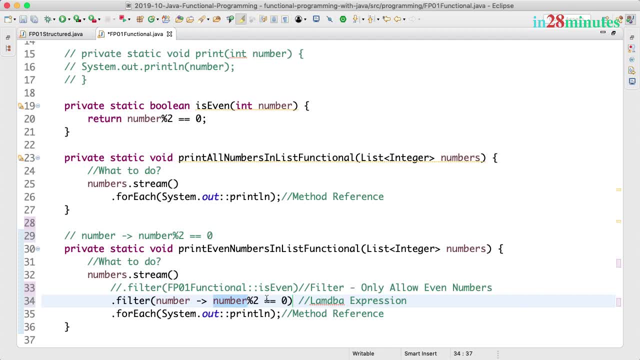 If number mod 2 is equal to 0, then return true back. Otherwise return false back. Let's see what would happen. No change in output, but you can see that now the code is much more simpler, because I don't really need to worry about this method anymore. 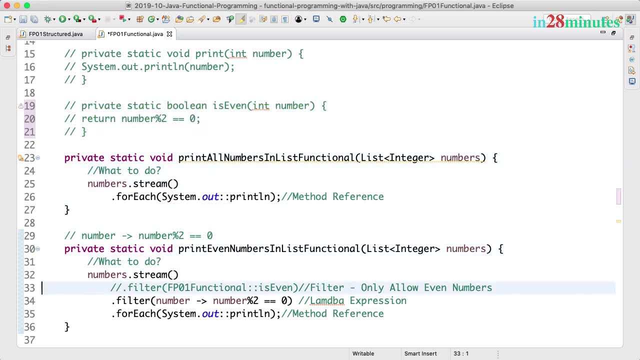 This method can be commented out- and all logic that we have right now. I'll move this line of code a little below. The logic that we have right now is to convert the list of numbers into a stream and, for each of the numbers, 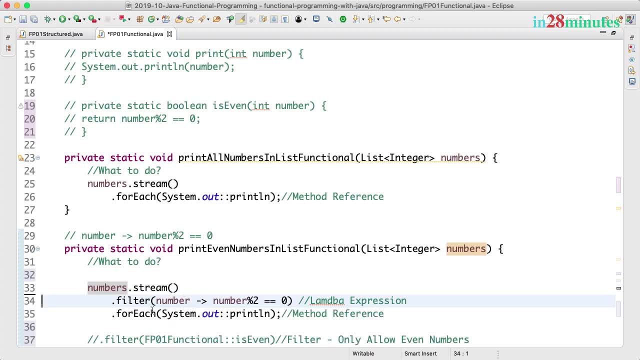 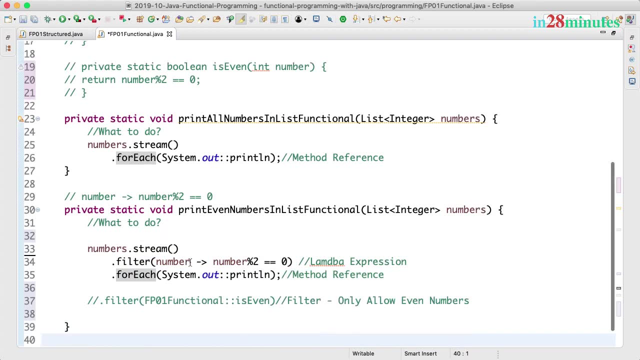 execute the filter. Is this condition true? If the condition is true, then go ahead and do the print. As you can see in here, with functional programming, we are focusing on the what to do For each element, what to check. 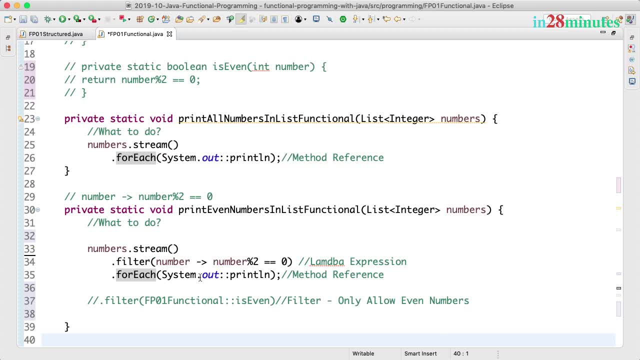 You are checking that the number is even For each element. what to do? if the condition is true, We want to print it out. What we learned in this specific step is something called a lambda expression. Lambda expression, as we discussed, is a simplified representation of the method. 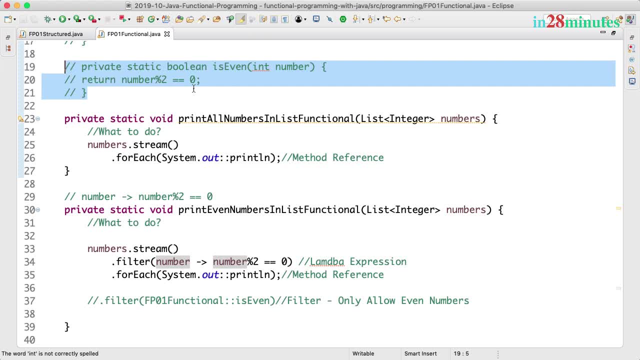 Over here we had a method called isEven, which was written in number. mod two is equal to is equal to zero. We just used the same logic in here in much more simpler syntax. If this is the first lambda expression that you wrote, 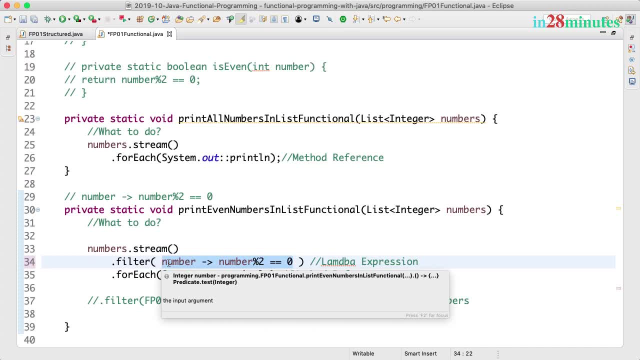 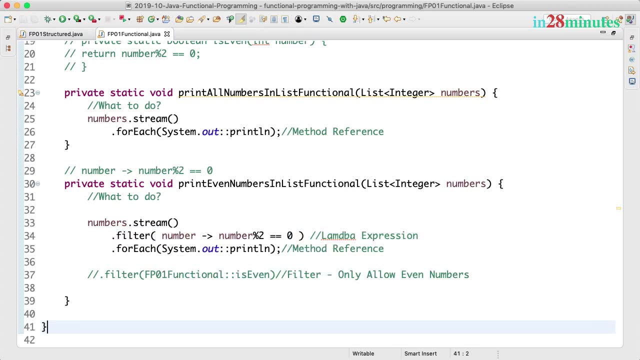 the syntax might look a little weird, a little new and all that, But don't worry, we'll be writing a number of lambda expressions in the subsequent steps and you'd really get comfortable with them. Let's quickly review the important concepts. 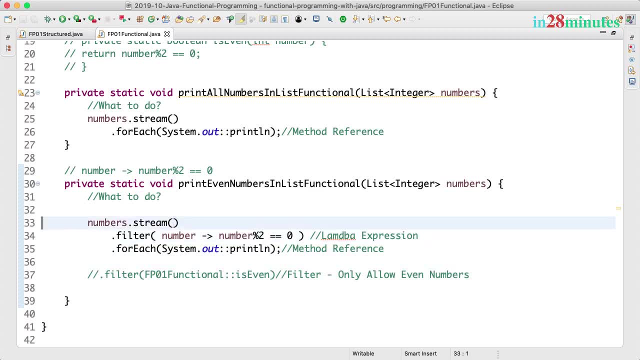 that we have learned until now. Number one: with functional programming, we focus on what to do. We convert the numbers into a stream and for each element in that stream we specify what needs to be done. A stream is nothing but a sequence of elements. 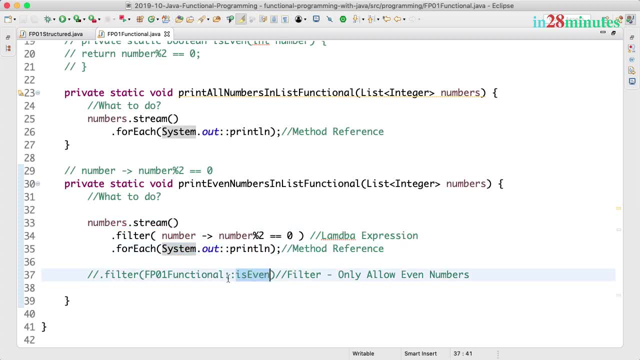 For each element. we would want to call the isEven method in here And we use a method reference to define that in here. The other approach to defining what needs to be done with each number is something called a lambda expression. With a lambda expression, 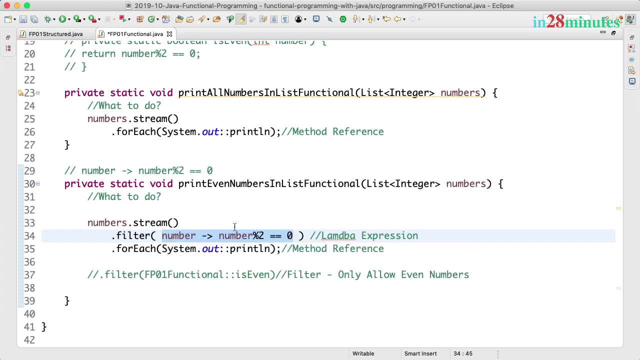 you can define the entire code directly in here. With a method reference, we are actually referring to a method which is defined somewhere else. However, with a lambda expression, we are actually defining the complete logic of the method right here. I hope you are having a lot of fun. 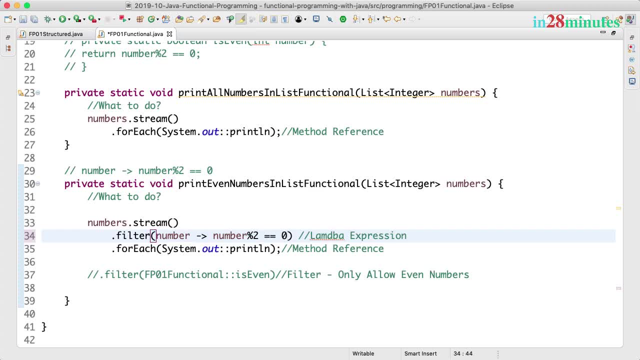 And I'm sure a lot of these concepts are new And, as I said earlier, FP functional programming is actually a paradigm shift, So it will take some time for you to get adjusted to this, So follow along and keep watching the next steps. 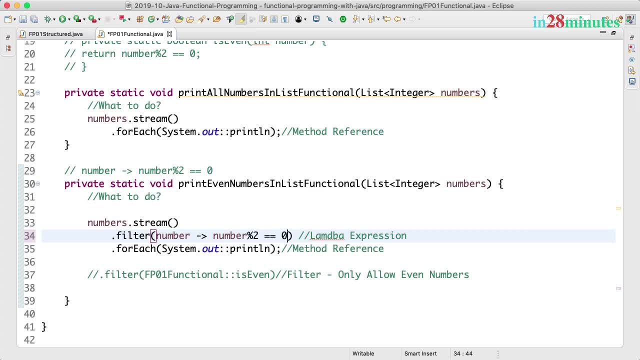 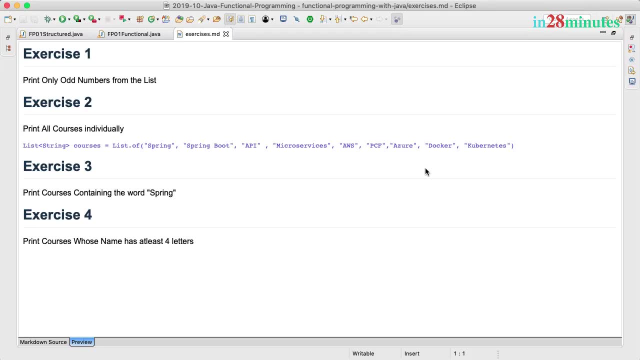 and I'm sure you'll be learning a lot about functional programming. I'll see you in the next step. Until then, bye-bye, Welcome back. In the previous steps we looked at a few functional programming basics, And in this step, 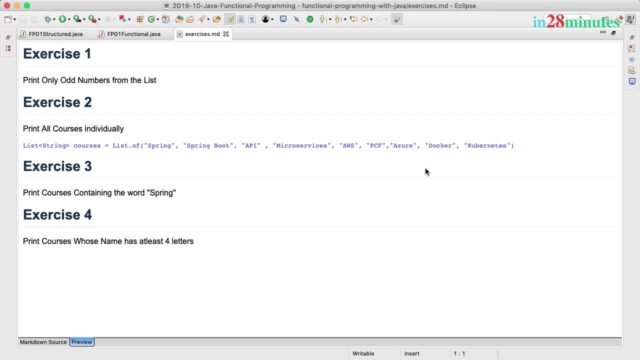 let's do a few exercises to try and consolidate our knowledge. Let's start off with a simple exercise. It's to print only the odd numbers from the list. So just like we have the method print even numbers in the list functional, create another method. 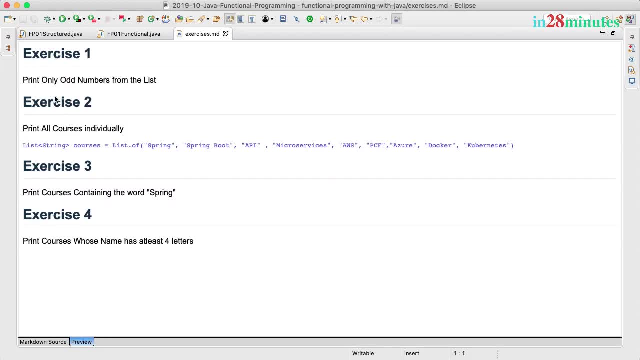 called print odd numbers in the list functional. The second exercise is to print all the courses individually Instead of using a list of integers. what we are doing in here is creating a list of string courses, and we are creating a number of courses in here. 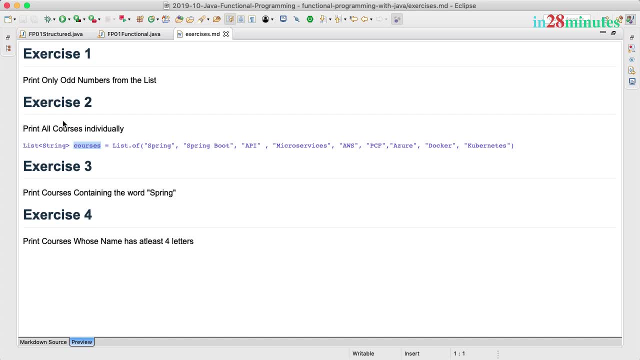 So we would want to actually take this list and print each course individually on its own line by using functional programming approaches. The third exercise is to print courses that contain the word spring. So print only those courses which contain spring in them. The fourth exercise: 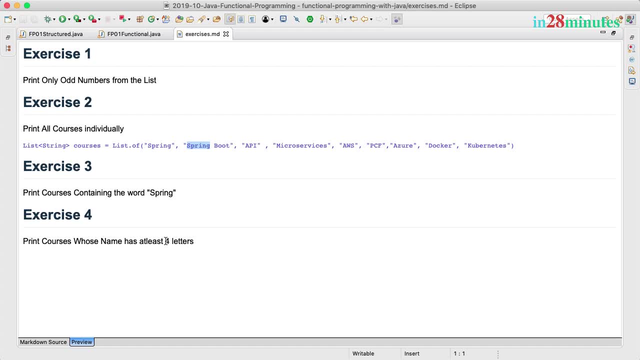 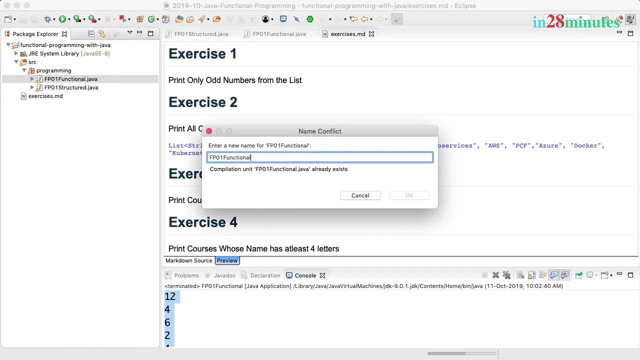 is to print courses whose name have at least four letters in them. You can pause the video in here and try these as an exercise. Now let's get started. I'll go to our FP01 functional copy it and I'll call this FP01 exercises. 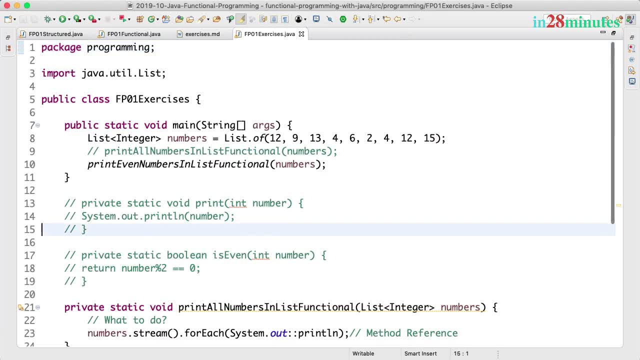 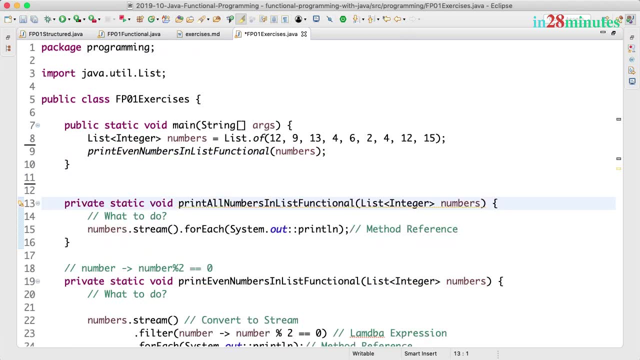 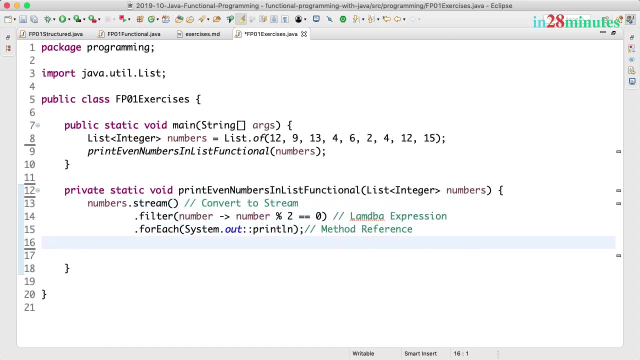 And over here. what I would want to do is to remove all the commented code out. So I'll remove all this stuff which is not really needed, And the only method that I'm interested in is to just print even numbers in the list. functional. 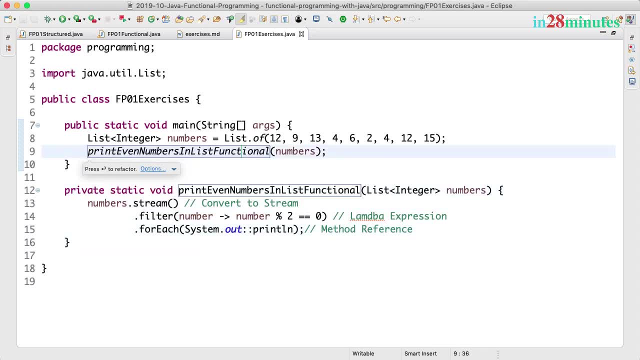 Cool, We have that ready. What we want to do is rename this Right-click refactor rename. Print even numbers in list. Actually, we would want to print odd numbers in list, right? How do I check whether something is odd? 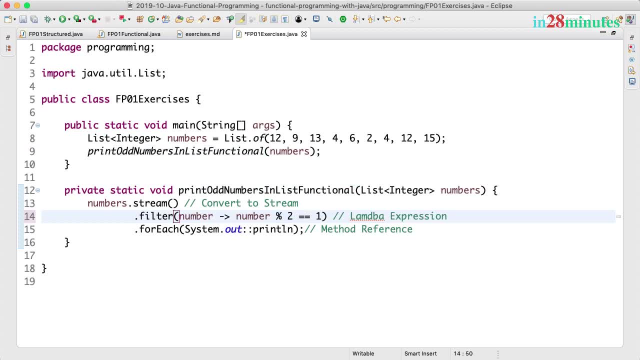 Number mod 2 is equal to is equal to 1.. So if a number leaves a remainder of 1, when divided by 2, it's an odd number, right? So that's basically the logic that we are using to print odd numbers. 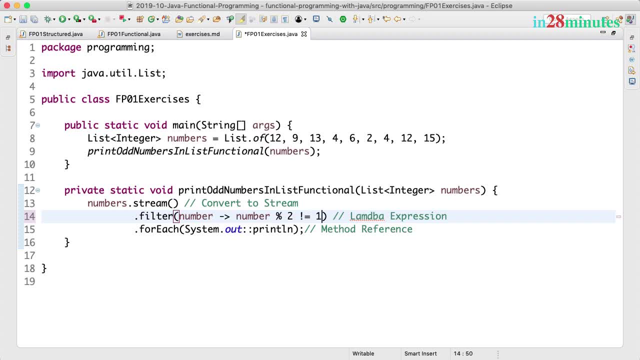 You can also say number mod 2 not equal to 0. Even this code would work. So is equal to, is equal to 1 or not equal to 0. Both of these logics should work, So I'll run this as a Java application. 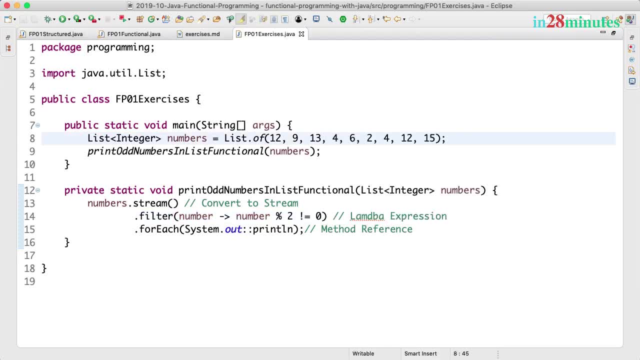 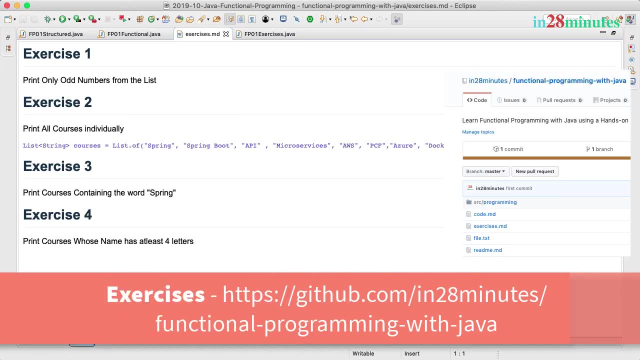 Cool 9,, 13,, 15.. So only the odd numbers which are present in here are being printed out. Now the second exercise was to print all courses individually. This should be simple, So what I'll do is, instead of creating separate methods for that, 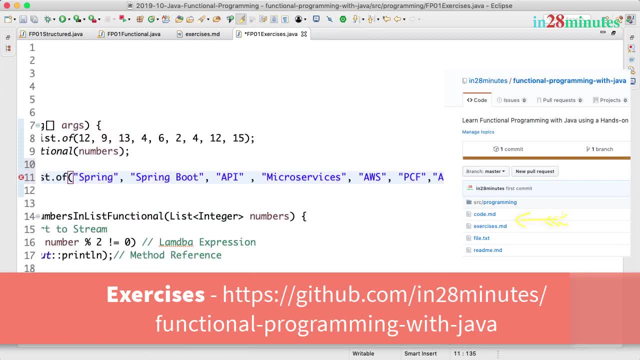 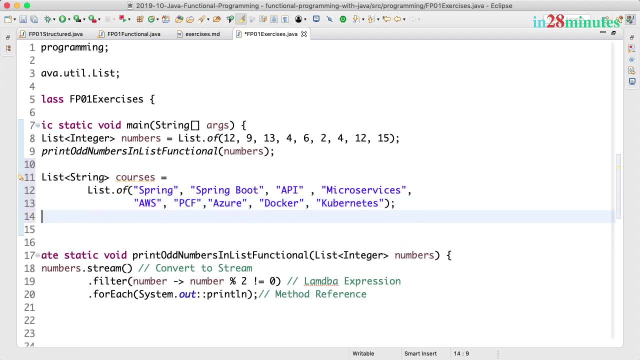 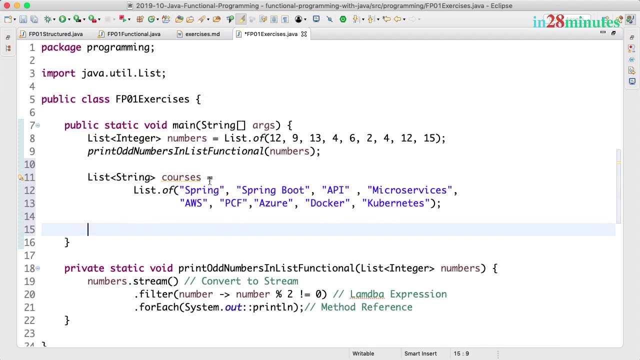 we'll actually directly write the code for it in here, So I'll create a list of courses. So if you look at these courses, there are quite a number in here. So Spring Spring Boot, API, Microservices, AWS, PCF, Azure, Docker and Kubernetes. 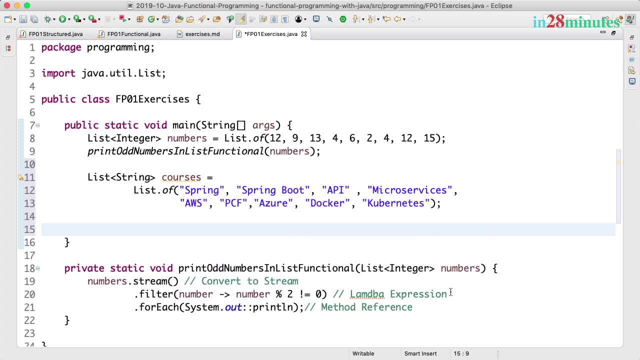 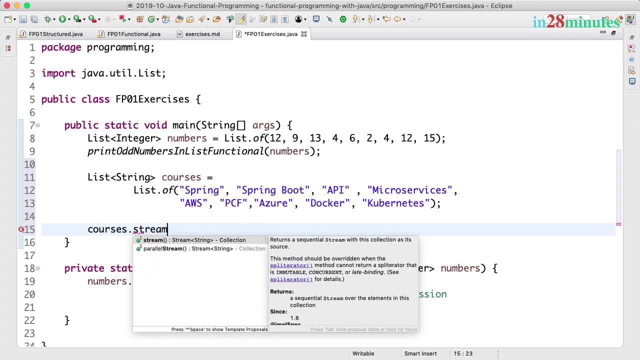 You can create a list like this, containing your favorite set of courses, And what we want to do now is we want to print all of them. So, with functional programming, the first thing that we would do is we will convert it into a stream. 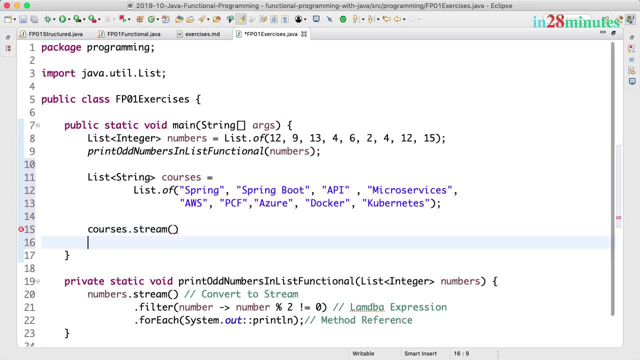 And for each element inside the stream. what do we want to do? first is we would want to just print out them. So systemout colon, colon, println. Cool, Isn't it easy? Let's comment the earlier one. So I'll comment these two lines of code. 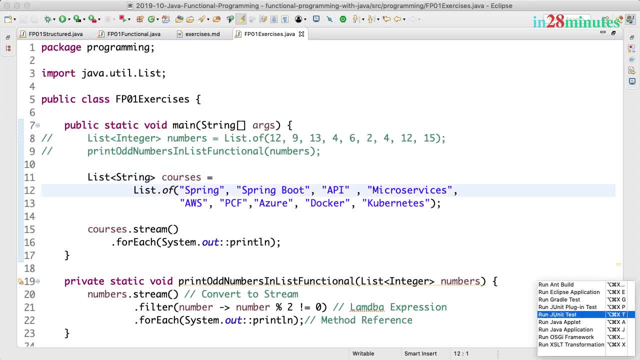 and let's execute just this line of code right now. Let's run it as a Java application and see all the courses that have been printed. So that's exercise two done. Now the exercise three was to print only those courses that contain the word Spring. 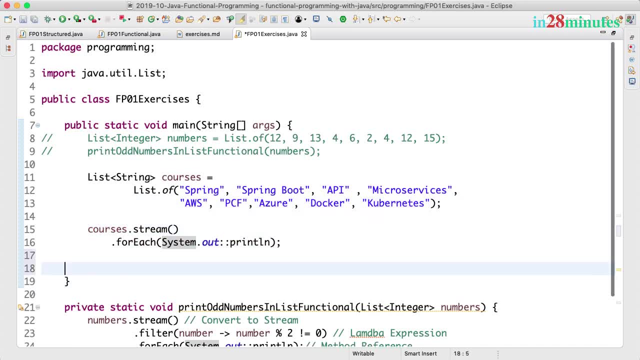 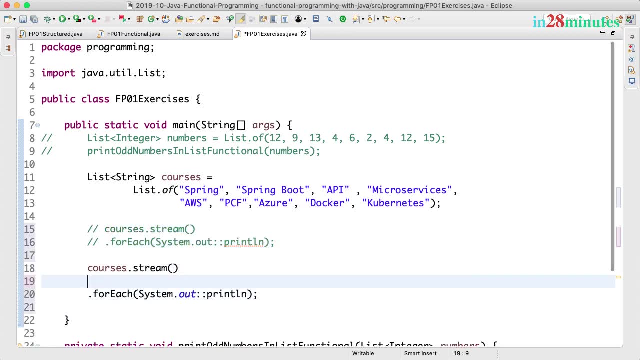 How do we do that? I'll copy this, paste this down, comment this out And over here. what we want to do is to add a filter, And what should be the filter For every course? only filter the course that contains the sequence Spring right. 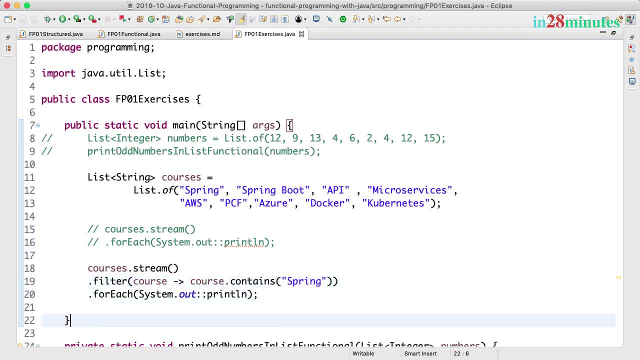 That's what we would want to do. Let's now try and run this Run as Java application Cool. Only Spring and Spring Boot are now being printed. Now you can pause the video in here and try the last exercise if you have not tried it yet. 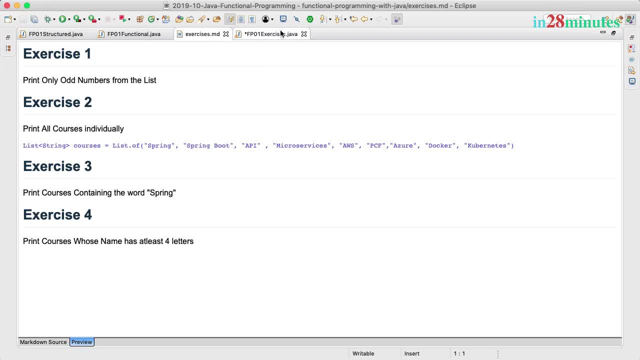 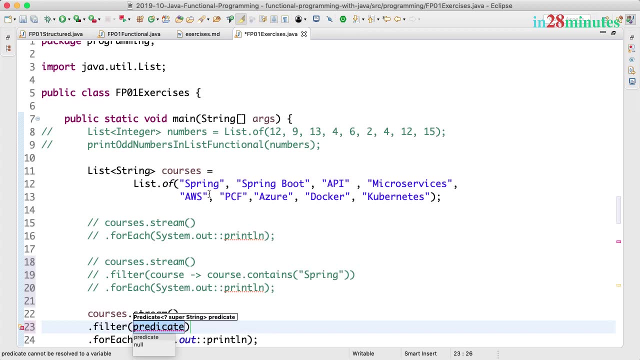 What's the last exercise Is to print courses whose name have at least four letters, So coursesstreamfilter. I would want to allow only those courses which have at least four characters, So I would want to eliminate AWS and PCF. How do I do that? 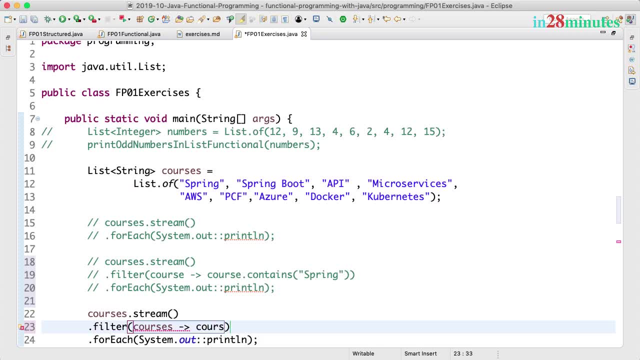 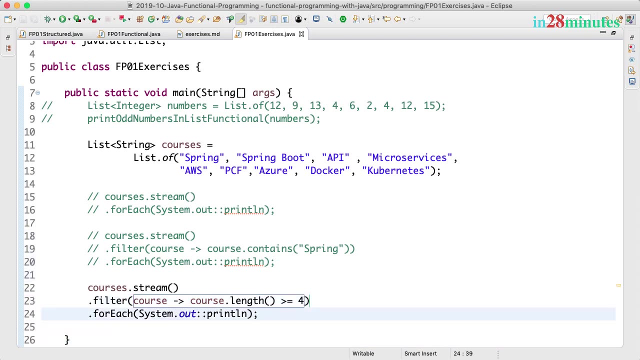 Over here I can define course and course. Oops, Actually I should use course in here, So it should not be courses. Courselength is greater than course length is greater than or equal to four. Now let's run this. 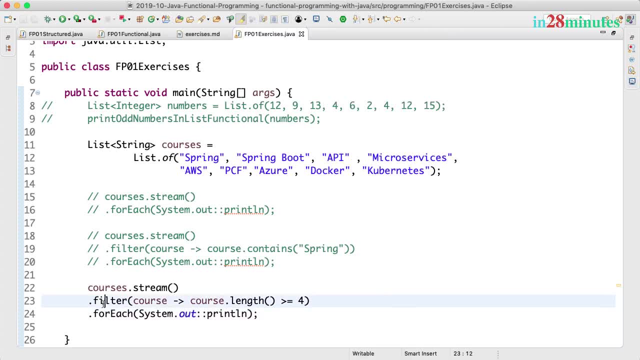 Awesome, Only six courses are being printed out, So you can see that now we are able to filter the courses that we would want to have. In this quick step we'll get a few exercises to implement the concepts that we have learned in the previous steps. 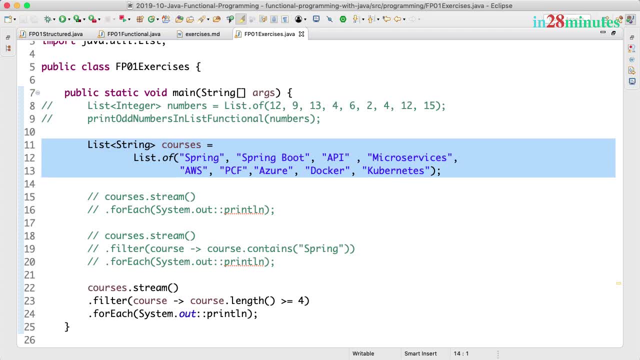 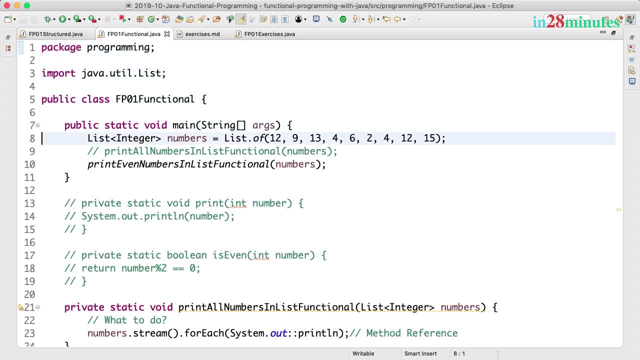 I'm sure you're having a lot of fun and I'll see you on the next step. Until then, bye-bye, Welcome back In this step. let's try and add a little bit more complexity into our functionality. What we would want to do is we would want to print. 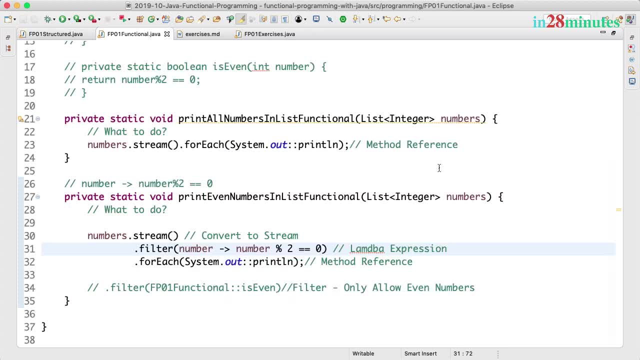 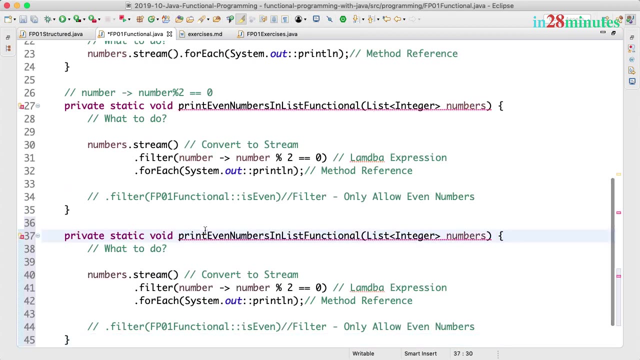 squares of numbers. Until now, we have been printing the numbers as is. How about printing the squares of each of these numbers? How do we do that? Let's look at that. So I'll copy this method out. I'll say: print squares. 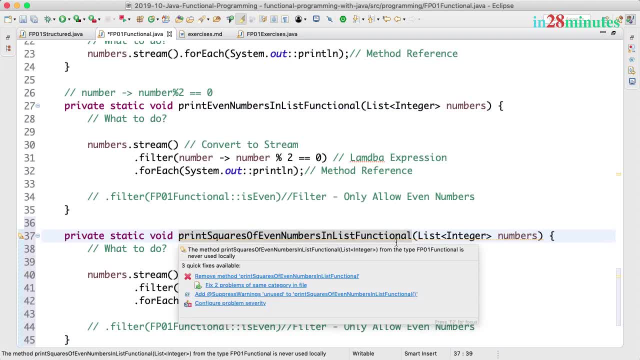 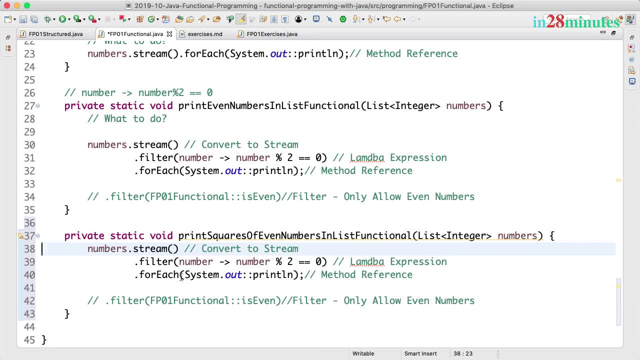 So let's print squares only of the even numbers in the list. So we have a stream. We are allowing only the even numbers to go through and then printing them. However, over here we would want to actually print the squares of the numbers. 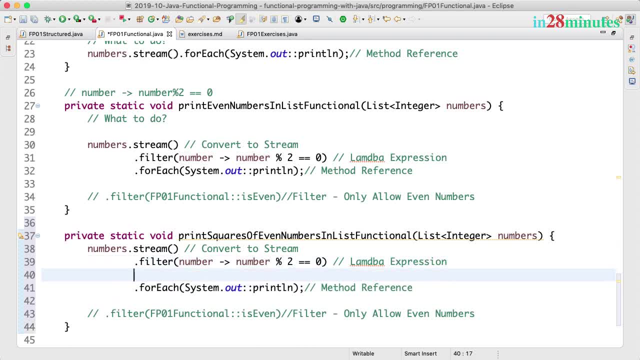 How do I do that? The way I can do that is by doing something called a mapping. So what we want to do is we would want to map each of the elements. We would want to take each of the elements and map it to the square of the element. 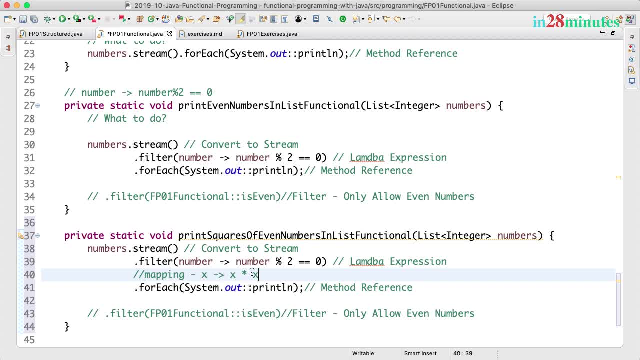 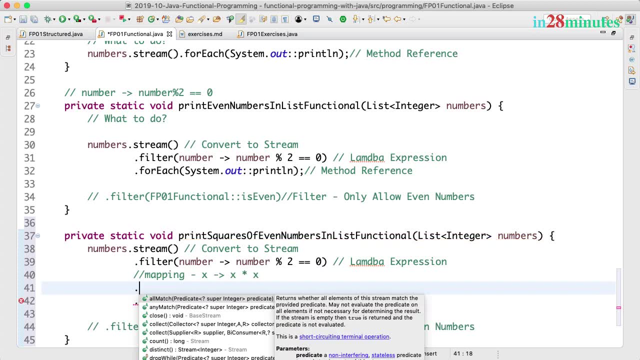 So we would want to calculate the square of each element and then print the square of the element. So how do we do the mapping? The way we can do the mapping is by saying map and you can define the mapper function in here, the mapper lambda expression in here. 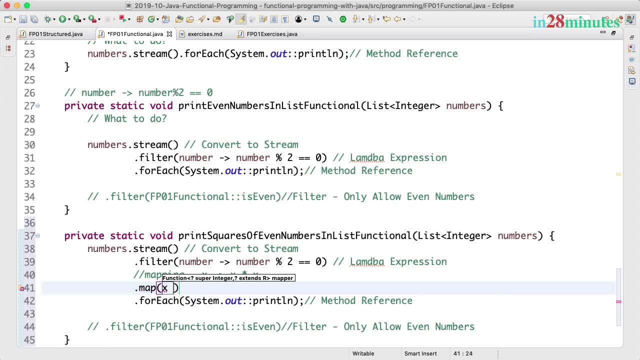 The mapper lambda expression is: take x or take any number, and once you have the number, what do we want to do with the number? We would want to actually multiply it by itself. So number, star, number. So this expression is called a mapping expression. 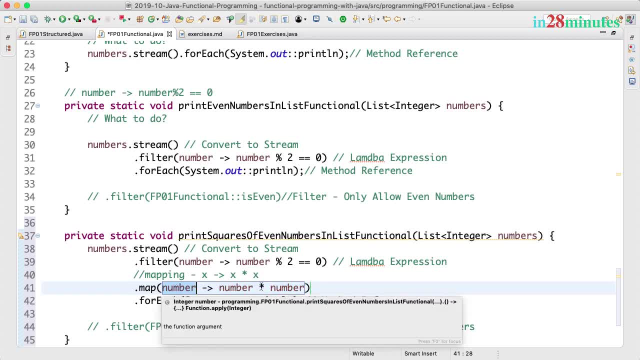 where we are mapping a number to number into numbers. The result of this is, at the end of it, the number would be multiplied by itself. So we'll calculate the square of the number, and after that the square would be printed. Let's try and run this. 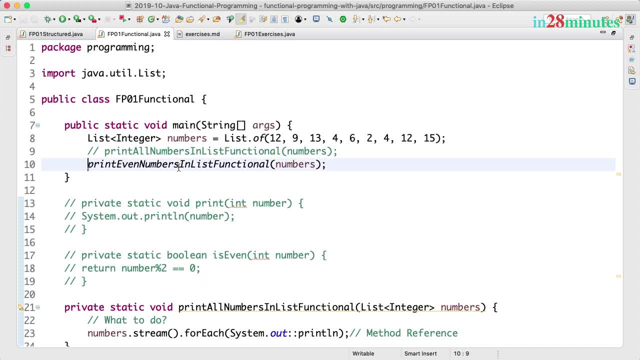 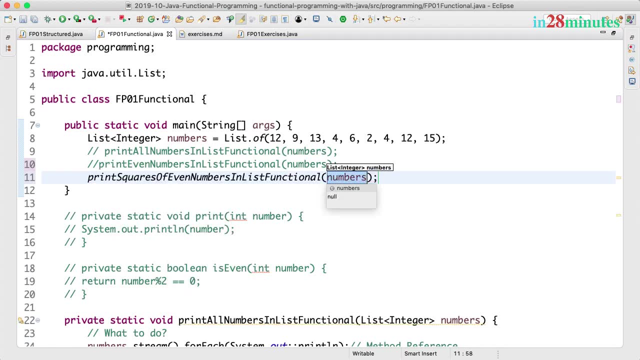 Oops, we have not changed the call in here, So we don't want to print even numbers in the list. We would want to print the squares of all numbers. So let's do this: Print squares of even numbers in list functional and let's run this. 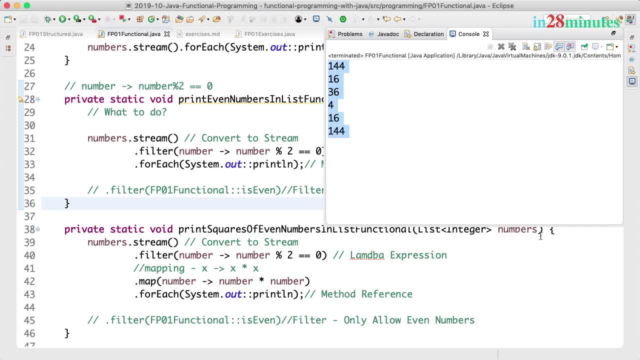 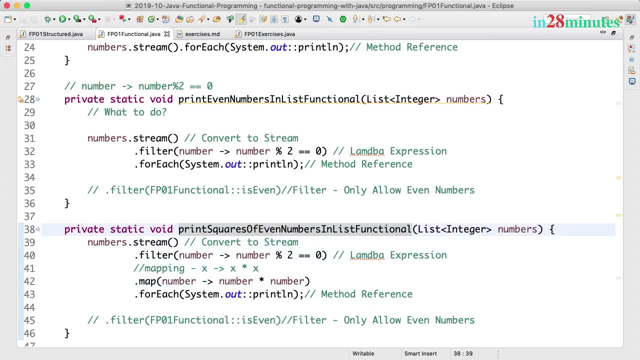 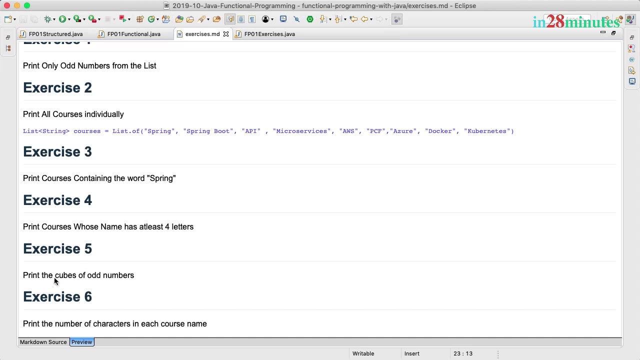 Run Java application and you can see that squares of all the numbers are being printed out. Now you can pause the video in here and try and do a few more things as an exercise. The two exercises are exercise five and exercise six. Exercise five is to print the cubes of only the odd numbers. 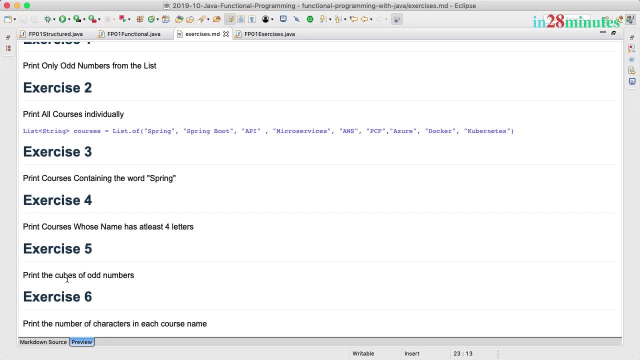 A cube is nothing but a number multiplied by itself three times. So three cube is equal to three into three into three, which is 27.. Exercise six is to print the number of characters in each course name. So I would want to print six characters. 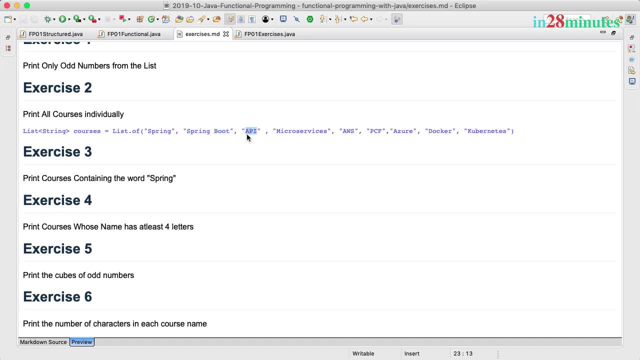 Here it would be 11 characters, Here it would be three. So instead of printing the course itself, I would want to print the number of characters in that. Now you can pause the video in here and try those two things as an exercise. 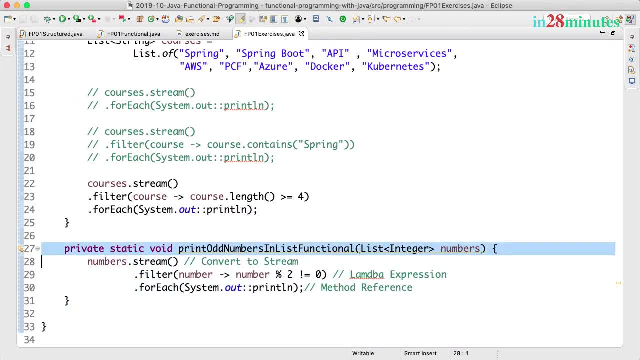 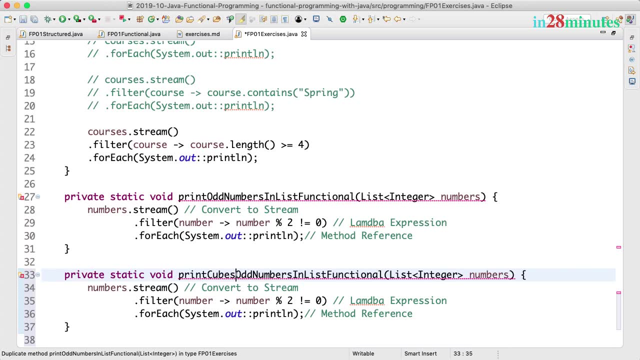 Let's go ahead and solve them. So what we would want to do in the exercises- I'm in fp01exercisesjava and what we want to do is print cubes of odd numbers- And the way I can do that is very simple, right. 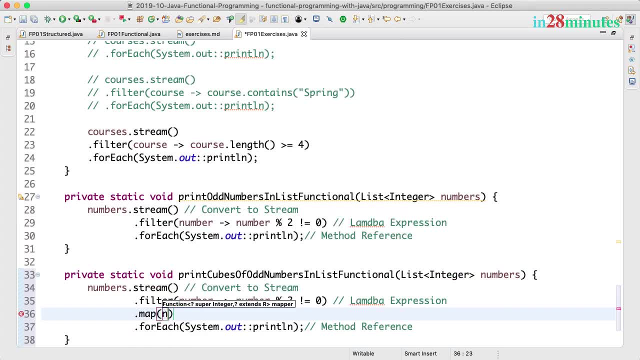 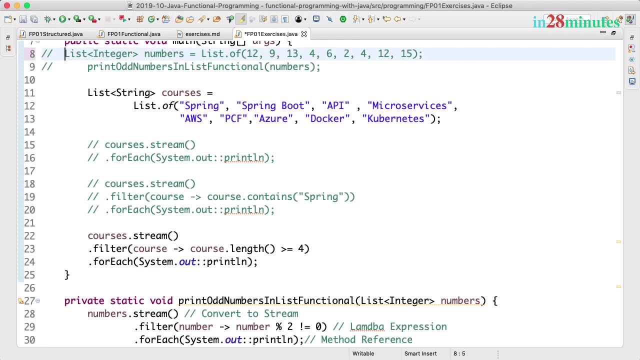 I would want to map each element, each number which is present in there. What do I want to do with it? I want to multiply by itself three times: number into number, into number. That's it. Let's take this and let's use the list of numbers. 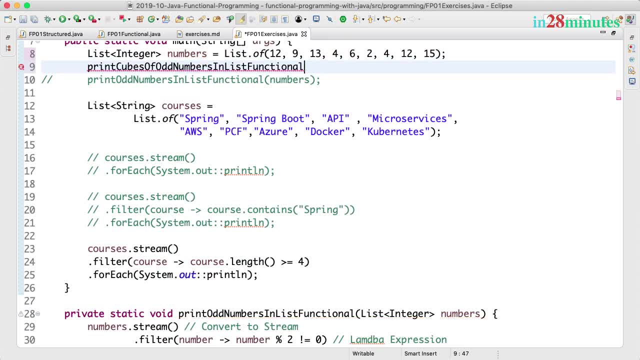 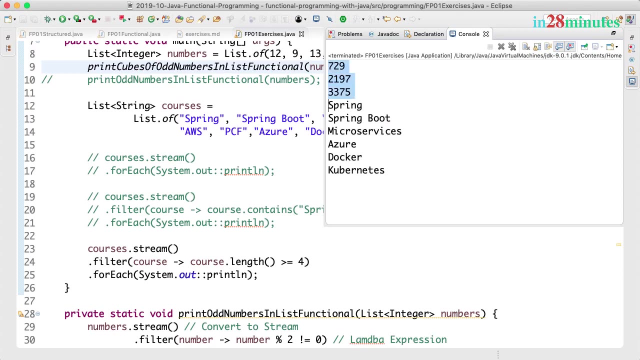 which we have already created, and call this in here by passing in numbers. Let's see what would be happening. Run Java application. The code is a little messy, So you can see that only for the odd numbers the cubes are being printed. 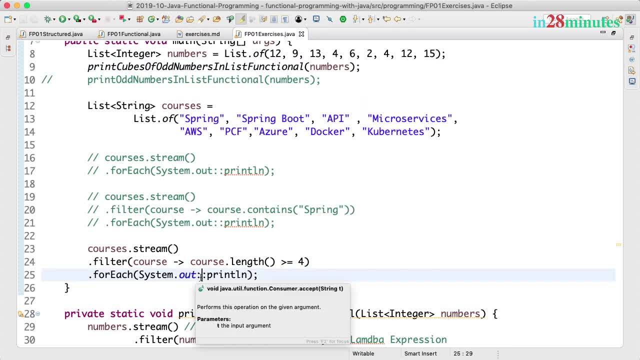 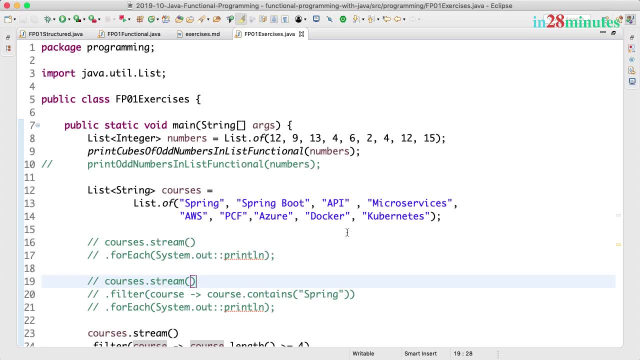 Don't really worry about what's printed after this. This is the result from the courses stuff which is after this, So that's good. We are now able to do the cubes of odd numbers. The next exercise was to actually print the length of these courses. 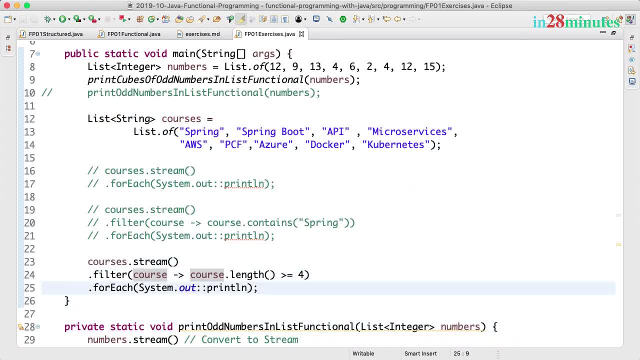 How do we print the length of these courses? Let's look at it right now. So what do we want to do? Coursesstream: We don't really want to filter anything For all the courses. what do you want to do? You want to print the length. 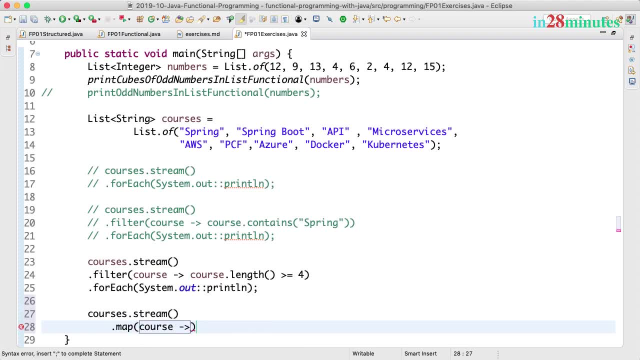 So we can map each of the courses. So each of the course. what do you want to map it to? You want to map it to courselength, So map course to courselength for each systemout. Isn't it cool? Let's not really worry about this. 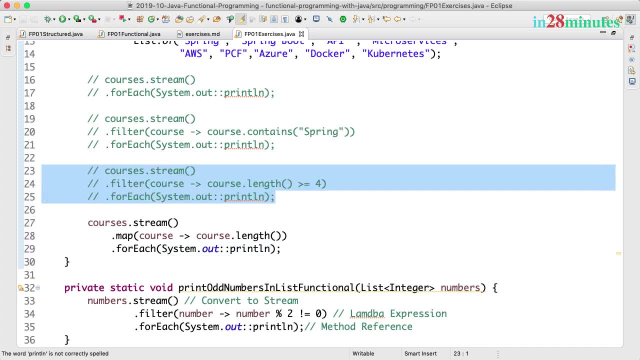 So let's comment this out And let's run this code. You can see over here that this is printing the lengths of each one of these, Just to be really, really clear. what we'll do is we'll append the course with a space and the courselength. 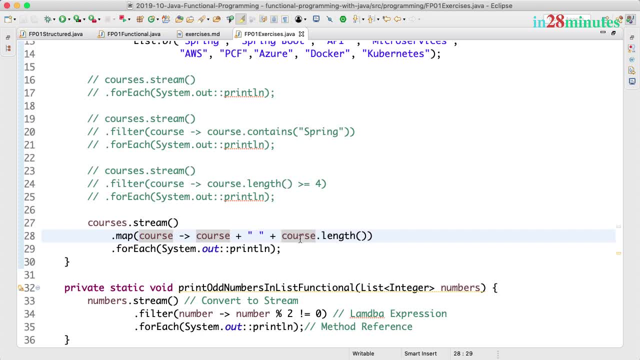 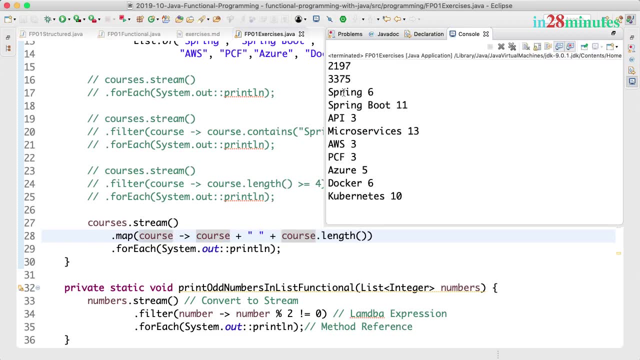 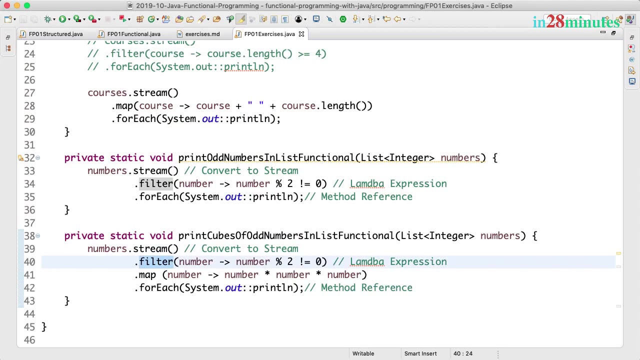 So what we are doing in here is course plus space, space courselength. Let's run this. You can see that it's printing spring six, Spring boot 11 characters, API is three characters, and so on and so forth, As we discussed before. it's very, very important. 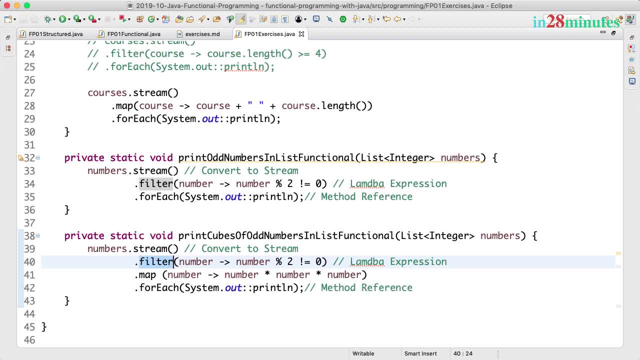 to get your hands dirty with functional programming. We are used to doing the traditional approach for a number of years And there is a lot of unlearning to do before we would get comfortable with functional programming. I hope you're having a lot of fun. 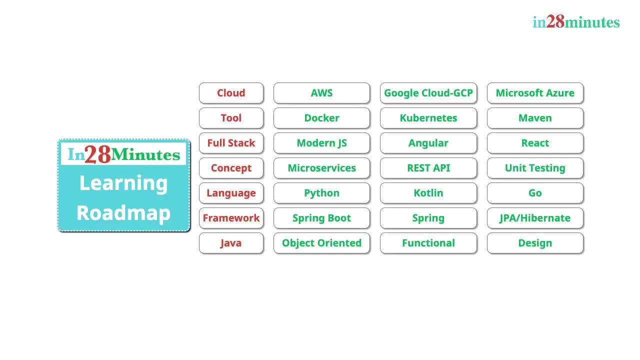 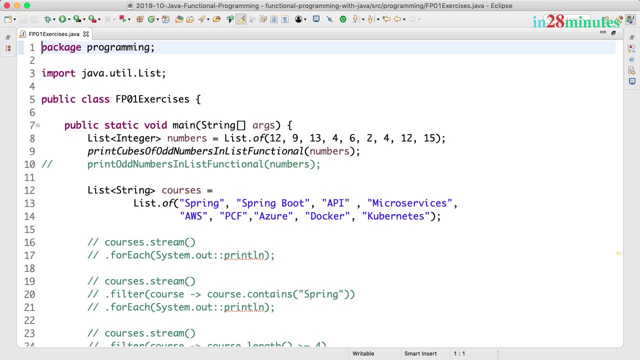 And I'll see you in the next video. Until then, bye-bye, Welcome back. Before we move into the next section, let's review some of the important concepts that we have learned in this specific section. The first thing that we have learned: 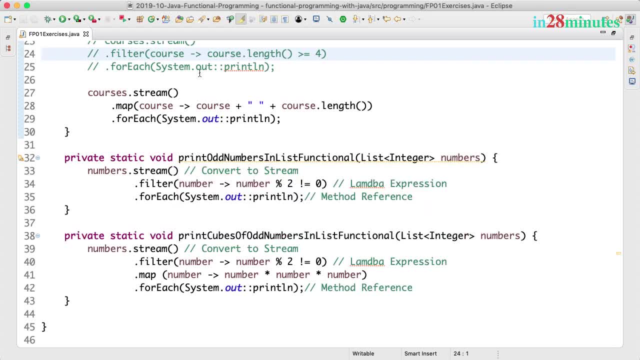 is in functional programming, we focus on specifying what to do. First of all, we converted the list to a stream, So this is a sequence of elements And for each element what should be done. Allow it If it's only an odd number. 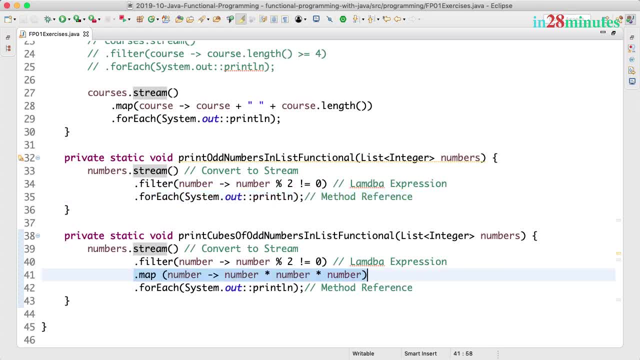 print the element out to the console, Do a cube of the number. So for each element in this stream we specified what needs to be done with it. We used numbersstream to convert a list into a stream, And then we looked at a couple of important methods. 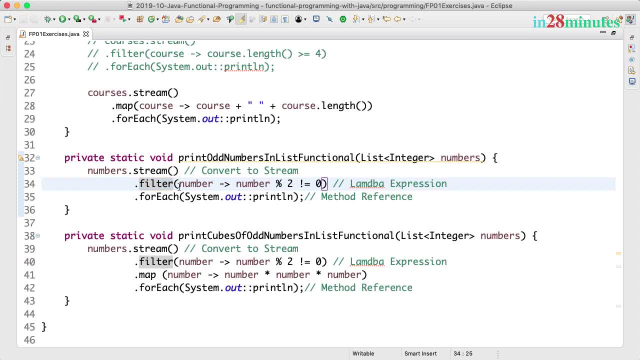 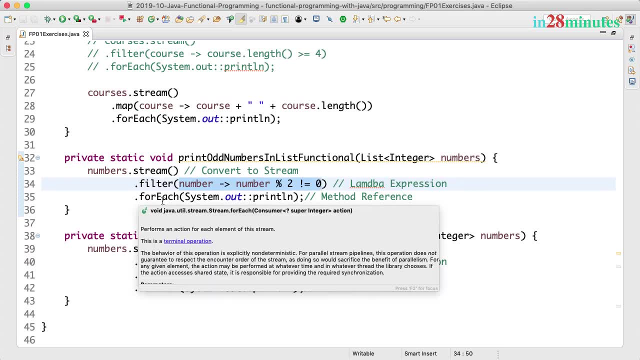 on this stream. We looked at filter, which allows us to specify a condition. Only if that condition is matched, then the element would go further. Otherwise, this element would be filtered out. So if I have a list of numbers and I would want to allow only even numbers to go through, 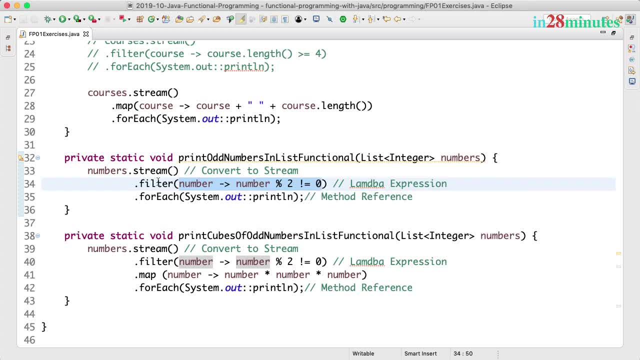 or odd numbers to go through. then I can define a filter specifying what is the condition that needs to be checked on. the number ForEach is used to consume an element. You take an element and print it. That's what this specific thing helps us to do. 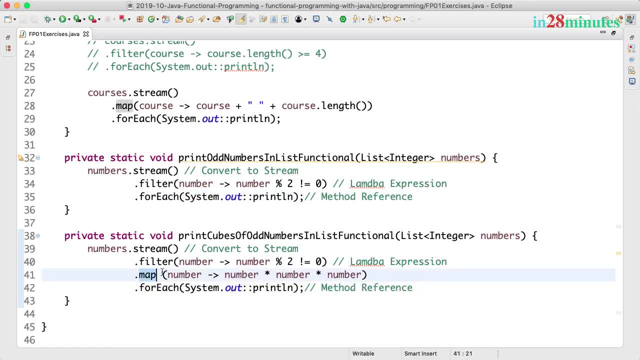 We used map to map one value to another value. So over here we took the number and we did a cube of it: Number into number into number. The other things which we looked at were lambda expressions. You can see that filter over here. 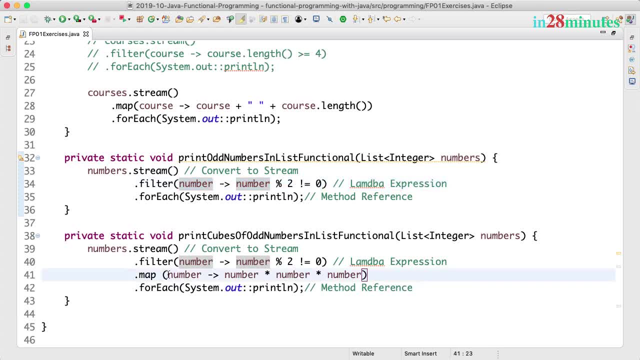 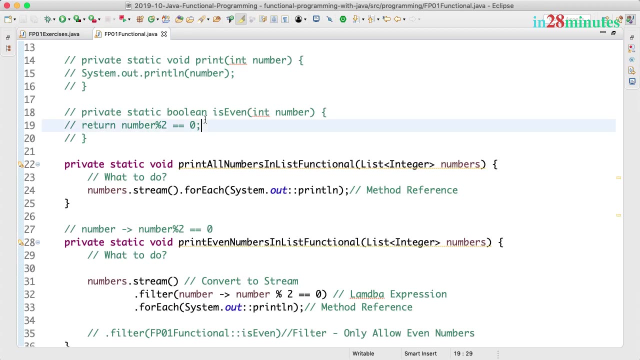 uses a lambda expression. The map over here uses another lambda expression. Over here we are using a lambda expression to take a course and append the course dot length to it. We learned that lambda expression is nothing but a simplified representation of a method.